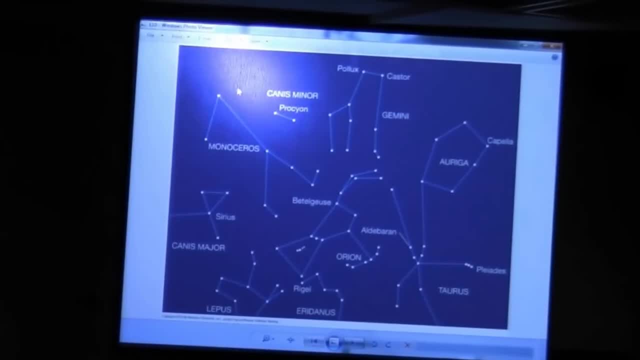 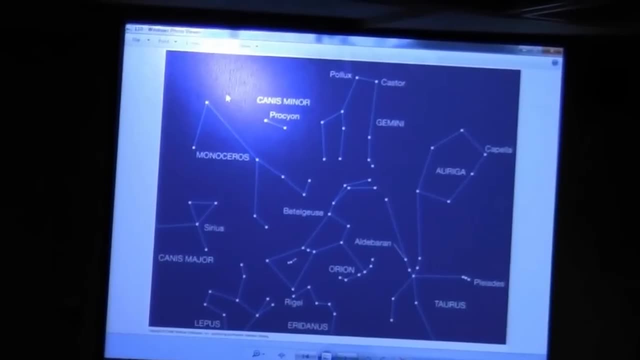 So let me ask you the question. We'll just do the basic question right now: How does this move over the course of the night? And to understand that we have to orient the room? So if we're going to orient the room, which way is north? That way, Franklin Street's. 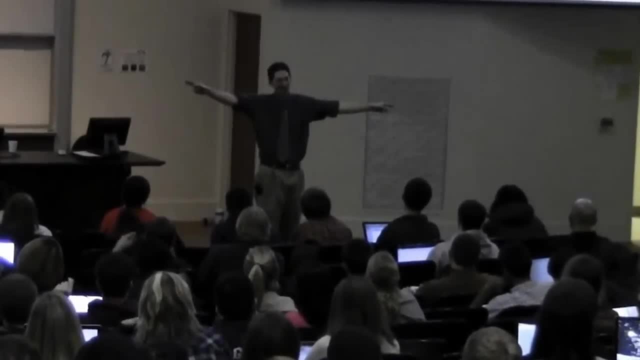 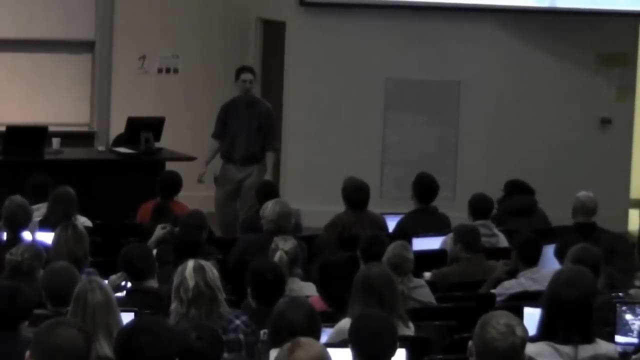 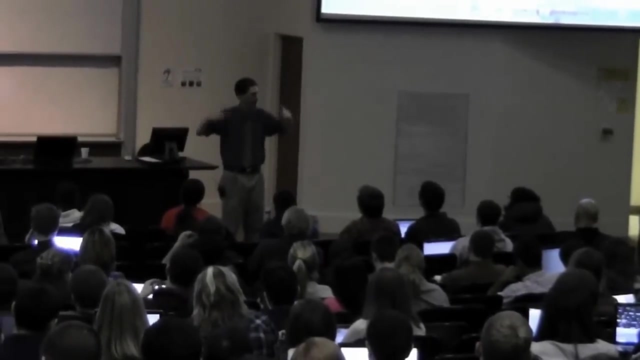 that way. That's not how I remember, And so south is that way. Which way is east Back there And west is over here? So in general, the stars rise where? In the east, In the west, And set in the west. So from our point of view, the celestial sphere rotates about. 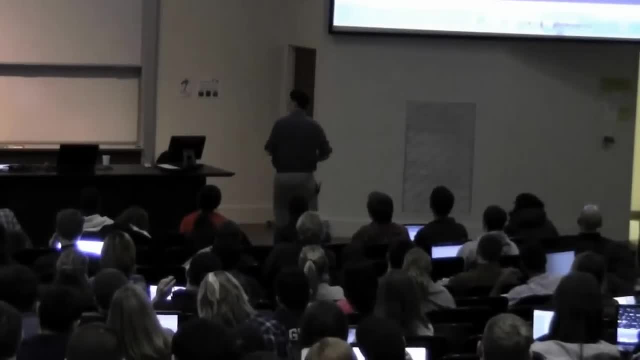 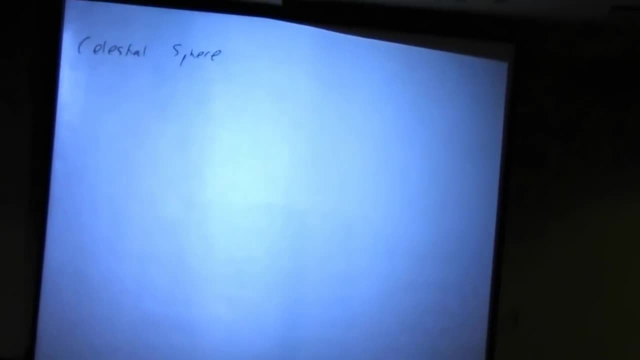 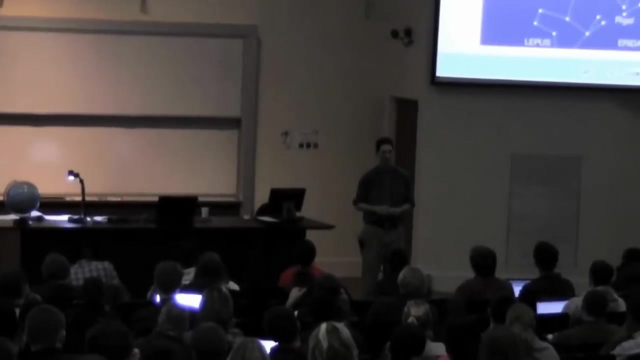 us. The ancient Greeks thought that's what was actually going on. But in reality, what's going on as we know today? Yeah, Earth is rotating underneath it. So if the celestial sphere is rotating from east to west, that means Earth is rotating from where to where. 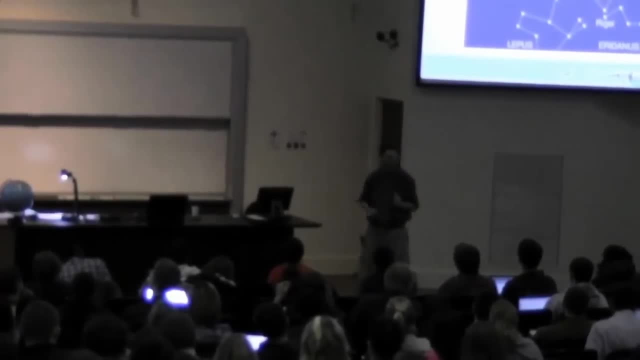 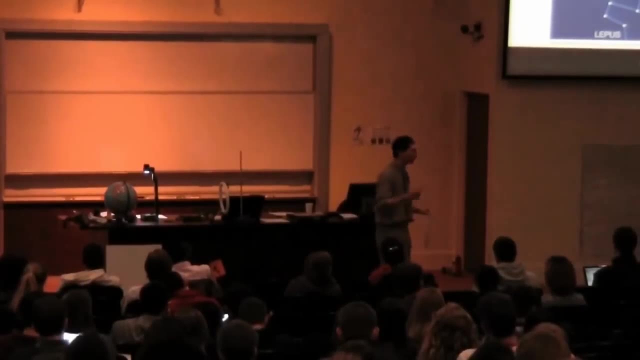 West to east. Okay, So we'll pick up with that next time. So if the stars are moving from east to west, we have two possibilities: The Earth is sitting here and the whole universe is rotating around us. Sounds crazy, but that's what they believed. 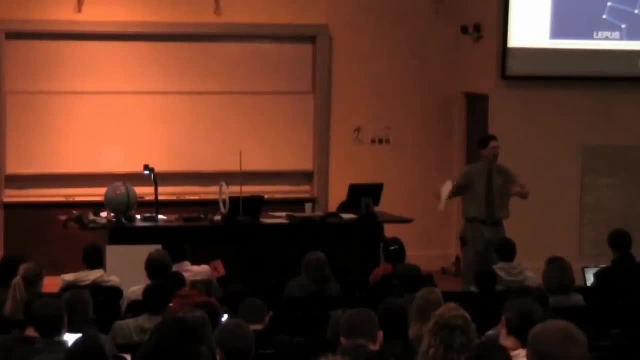 for thousands of years. That's the ancient Greek model, Or the stars are out there and Earth is just spinning on its axis. We all now know in the modern day that's the case. But back in ancient times, ancient Greek times, it was a reasonable idea to think that the 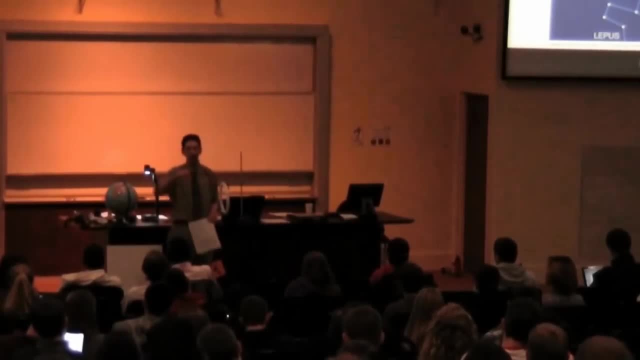 Earth is stationary. I mean, if you're on a merry-go-round, you feel the rotation right. You want to be thrown kind of to the outside. Or if you're on a track driving your car or some vehicle, you're kind of pushed to the outside. Do you feel Earth's rotation? No, you don't really feel. 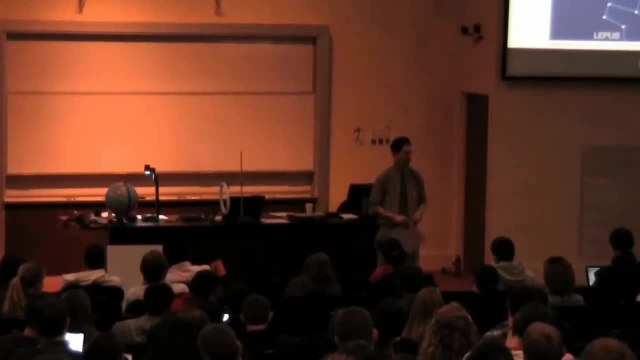 it. But there is a force It's called. you do have the same kind of feeling. You are being pushed slightly to the west. I think it is. It's called the Coriolis force And we'll talk more about it in lesson two. But if you crunch the numbers, the size of the 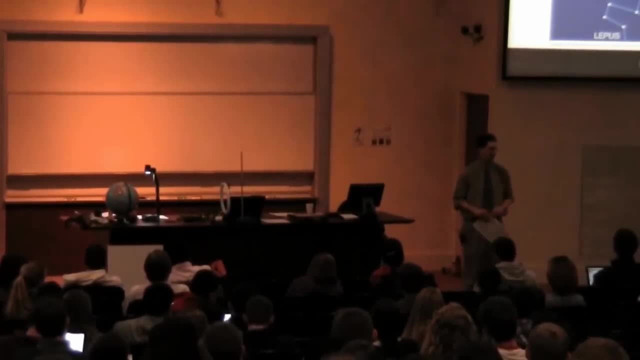 Earth and the rate at which it's spinning, the force that's inferred from that. it's small compared to the force of gravity. So gravity is our attraction to the center of the planet, all the masses beneath our feet. Gravity is an attraction between masses. So we have this. 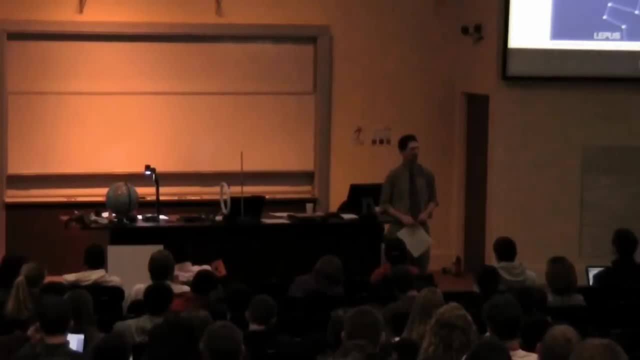 pretty sizeable force pulling us down, So don't really notice the small force pushing us to the side, the Coriolis force. So back then it seemed a very natural idea that Earth is stationary. Also, we kind of like, historically, psychologically, we like to think that Earth is stationary. So we kind 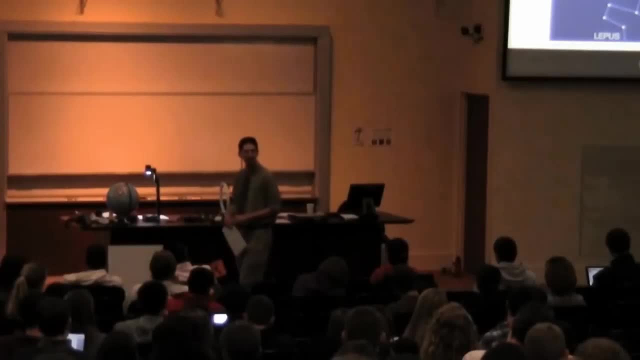 of like: historically, psychologically, we like to think that Earth is stationary. So we kind of like: historically, psychologically, we like to think that Earth is stationary. jZ, jZ, z, jZ, jZ, jZ, jZ, jZ, jZ. 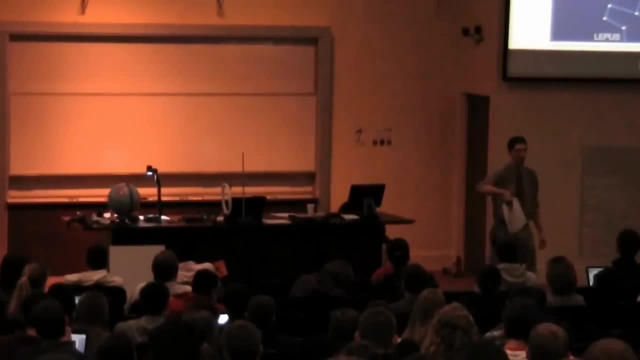 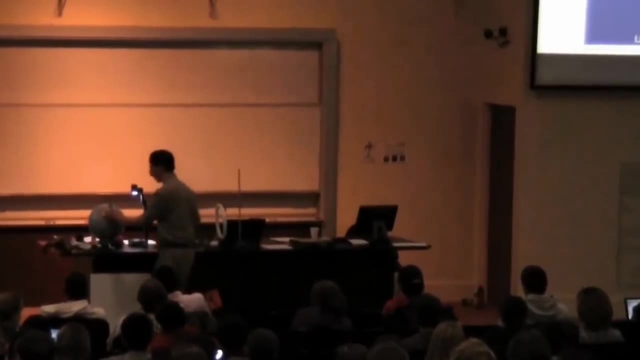 And if the stars are going from east to west, that means Earth is rotating. in which direction? West to east, the other direction. So we can do it a couple of different ways. Here I have a globe that we can use for different things and we'll use for different things. 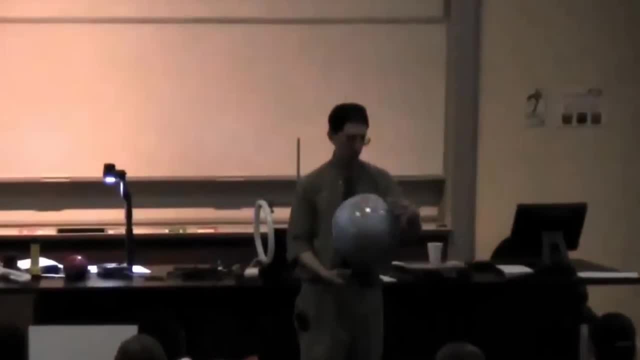 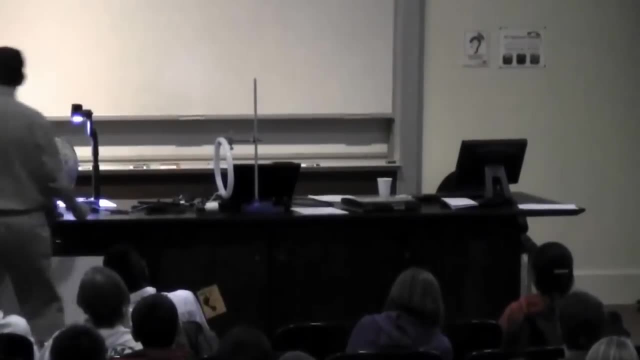 And I've already busted it. There we go, And so the globe west to east. well, it's kind of hard to see. So let's not use the globe. I mean for those in the back. you really can't see the details on the globe. 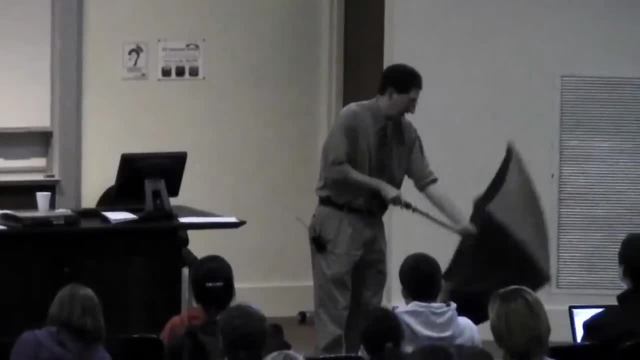 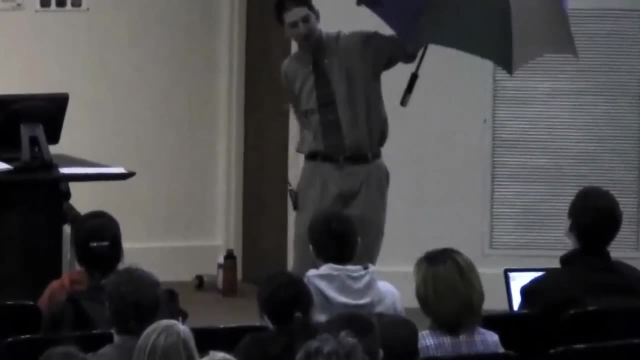 So let's use an umbrella instead. You can think of it. we can use this for many things. We can think of this as part of a globe like. this is the northern hemisphere of the globe. You can just envision the rest of it down beneath. 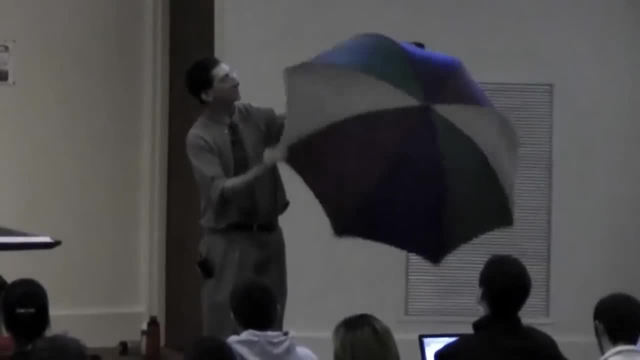 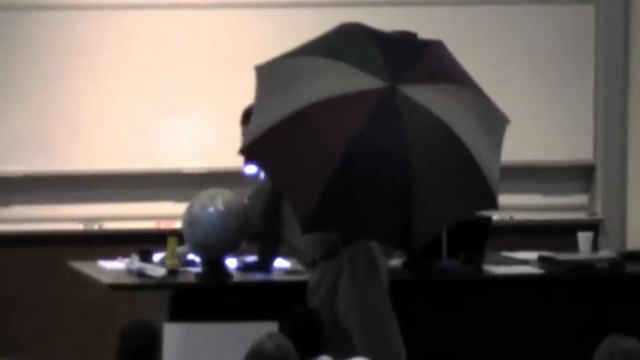 Use your imagination, And so let's pick some area to be the United States. So here's the United States, And so we've got a west coast and an east coast. I'll just mark it with sticky notes that I brought and spilled water on, so, hopefully. 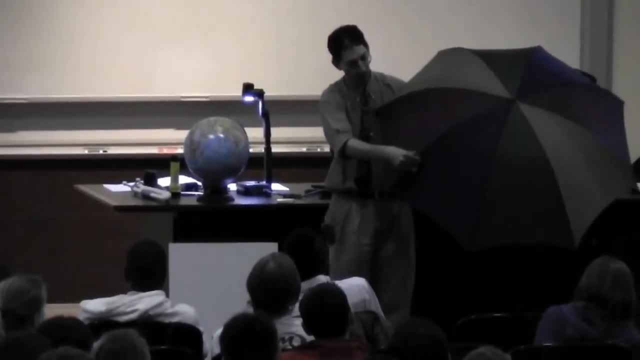 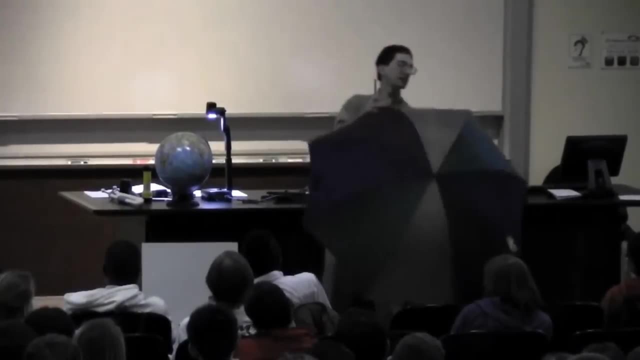 they still work, Okay, So, So let this be the west coast of the United States. so maybe that's LA, And there go my sticky notes. And where is it? This would be the east coast of the United States. so this is New York. 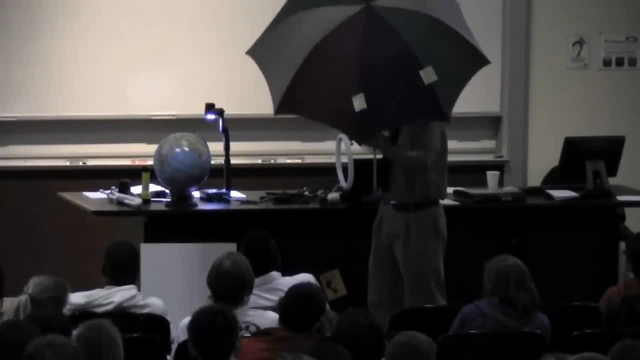 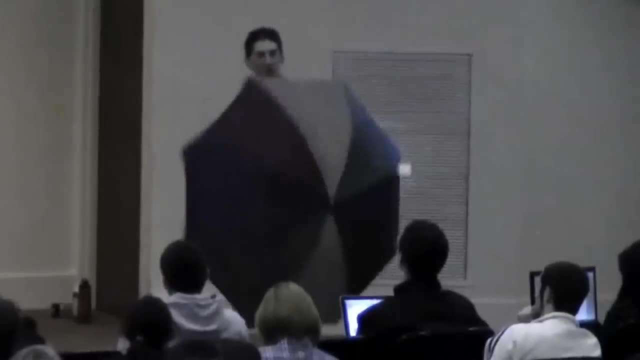 So west to east motion, that means we're going from LA to New York. so this direction, So this is the direction that the Earth spins, Is that clockwise or counterclockwise? Counterclockwise- Is it clockwise or counterclockwise? 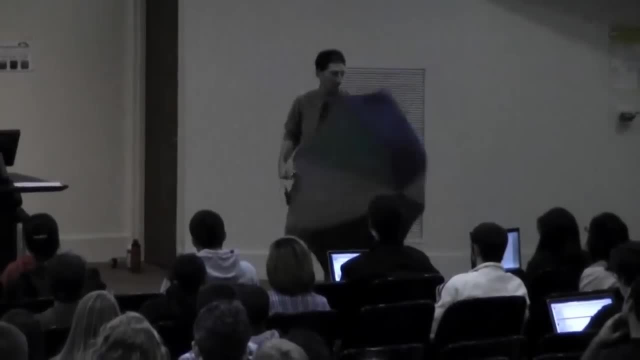 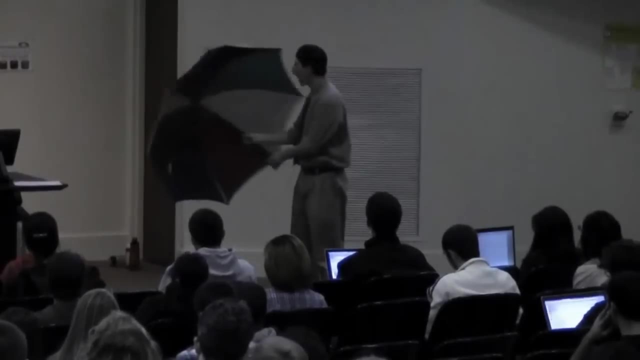 Clockwise, It's counterclockwise. So when we say the Earth spins counterclockwise- and that's how we normally refer to it- we're talking from as viewed from a particular direction. If we view it from down underneath the Earth, it appears clockwise. 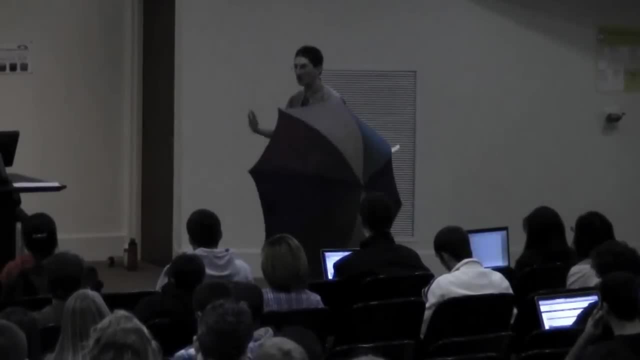 If we view it from over top of the Earth. by over top I mean if you ran up to the North Pole and jumped out into space and then looked down, it'd be a counterclockwise rotation. It's important to define that, because the solar system, all the planets, are in a plane. 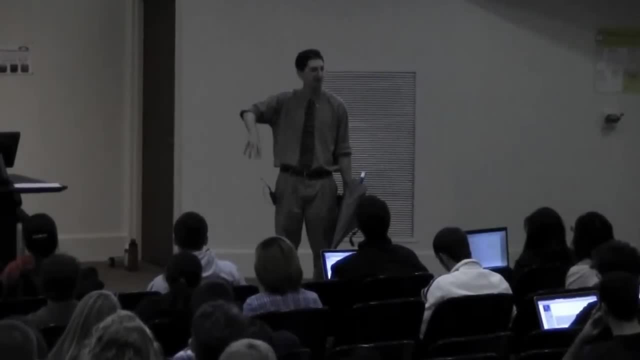 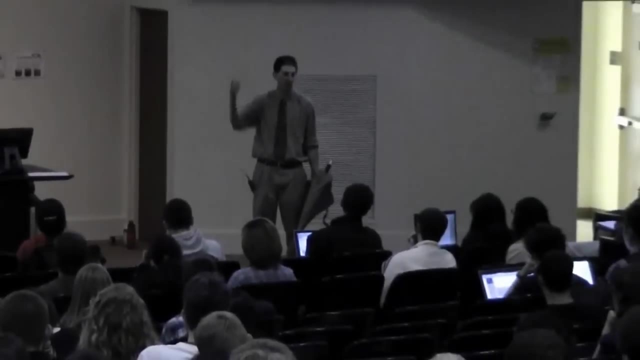 And all the planets, for the most part, are in a plane. There are some exceptions. They all rotate in the same direction. They all orbit around the Sun in the same direction And so, as viewed from the top of the solar system, over top of the North Poles of all, 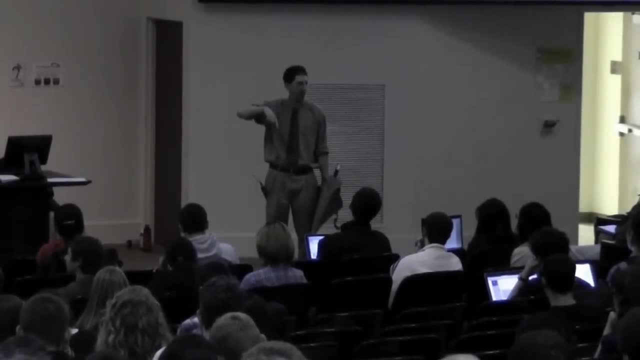 the planets, at least, approximately everything seems to be moving counterclockwise. Even the Sun rotates on its axis counterclockwise, But from the bottom of the solar system. there's no top or bottom in space, but we can define. 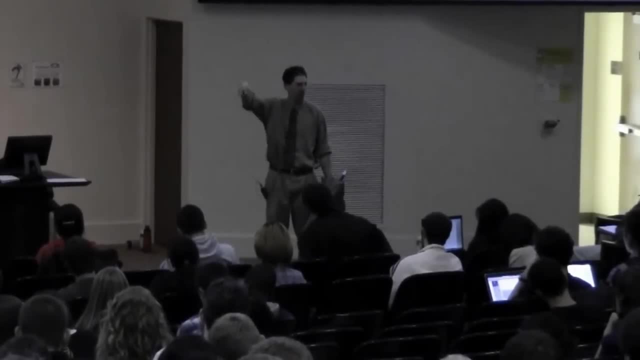 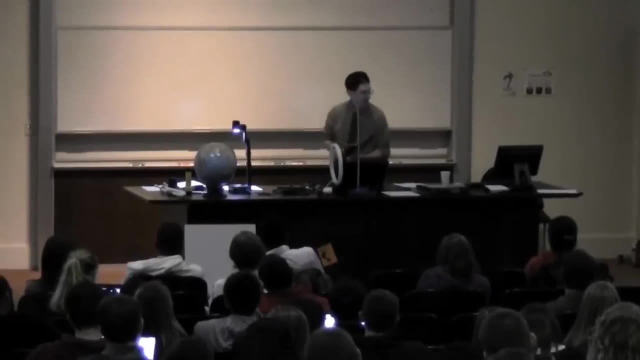 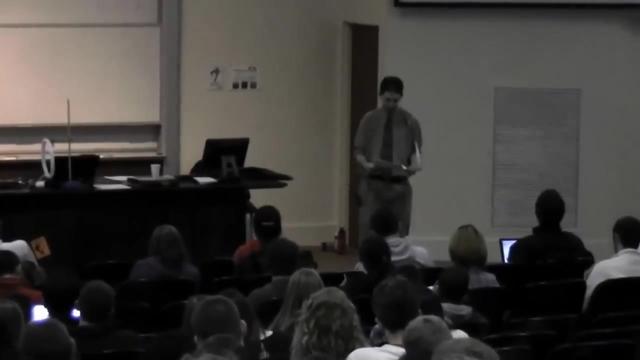 one plane of the solar system. Everyone go to their North Poles and jump off and look back down. It's a counterclockwise motion. So that's just something good to keep in mind. Let's see. Okay, so the Earth rotates counterclockwise as viewed from the top down. 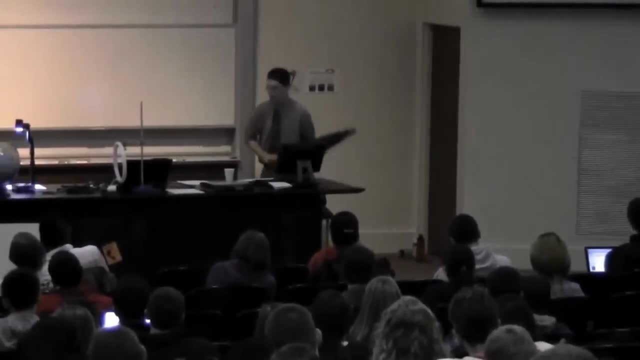 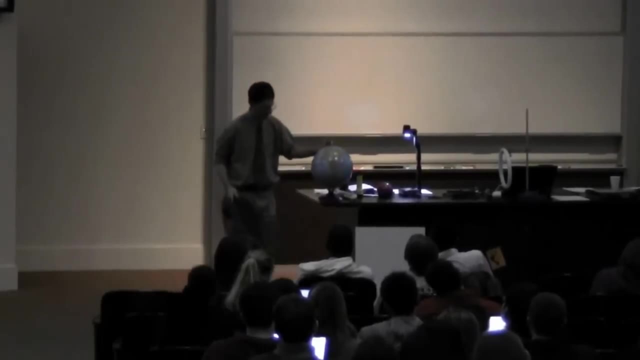 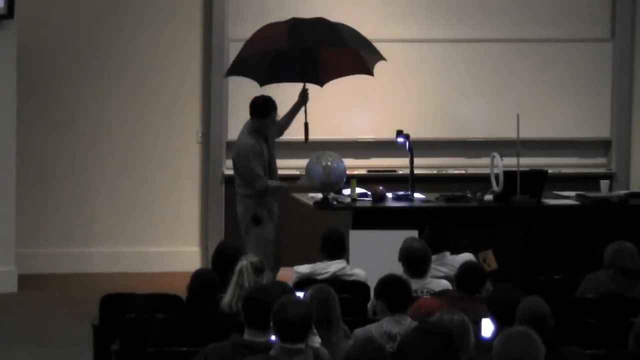 So okay, So Earth is rotating counterclockwise. Maybe we'll use both the globe and the umbrella. The globe can be the Earth, And now we'll let the umbrella be not the Earth, But the celestial sphere. So I'll just extend. 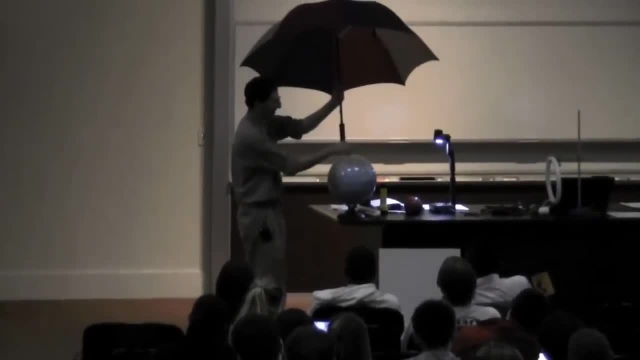 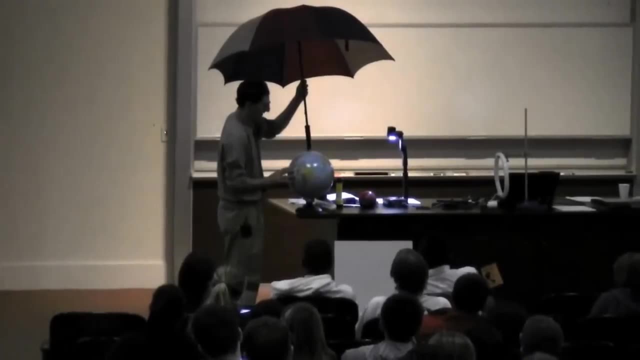 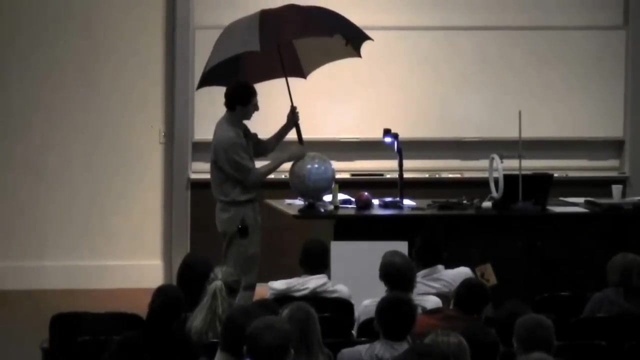 Here's Earth. It has a rotation axis And I'll just extend that axis with the shaft of the umbrella here. Now Earth is rotating, I'll get it going the right way: west to east. So that's in this direction. So, and the sky, as we said, not in the ancient Greek model, but modern day realization is. 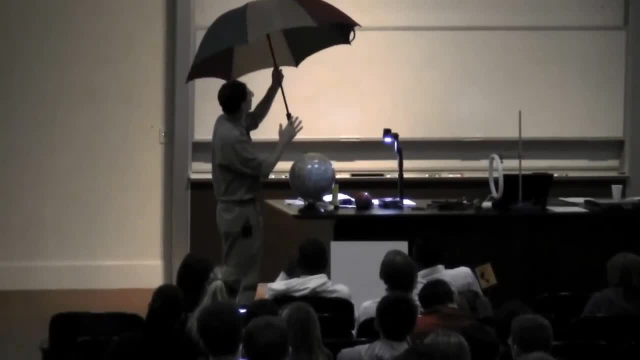 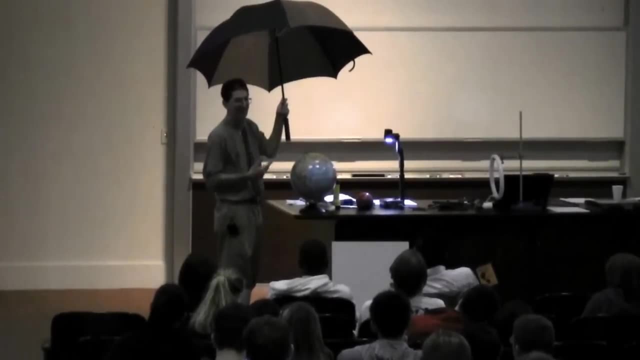 the sky is just standing there. Again, we talked about the celestial sphere. We can envision all the stars as painted on a sphere That encompasses us. It's not reality, But since we can't see distance, it's equivalent. So let's keep our construct of the celestial sphere. 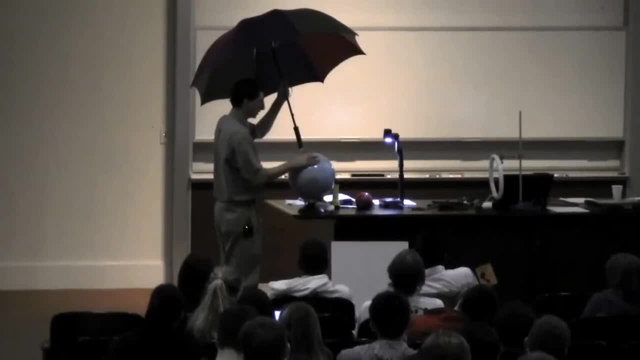 Here's Earth rotating underneath it. Now, from the point of view of someone on Earth, as I said, we don't feel our rotation. So it's equivalent to say: Earth is standing still and the sky is rotating in the other direction. Here we're going around. yep, that's counterclockwise from the top. 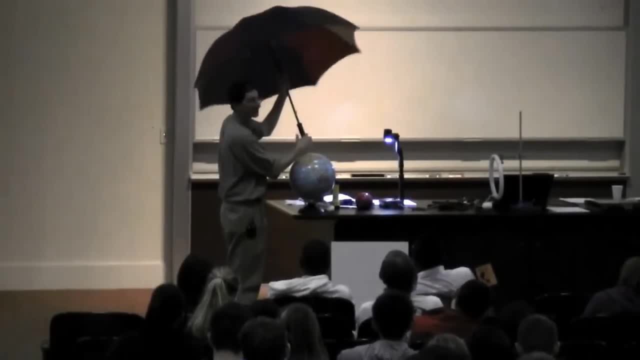 So we can equally think of us standing still and the sky rotating around us Make sense, Okay, So my question to you: is there a point in the sky where the stars do not appear to move as viewed from Earth? Yes or no? 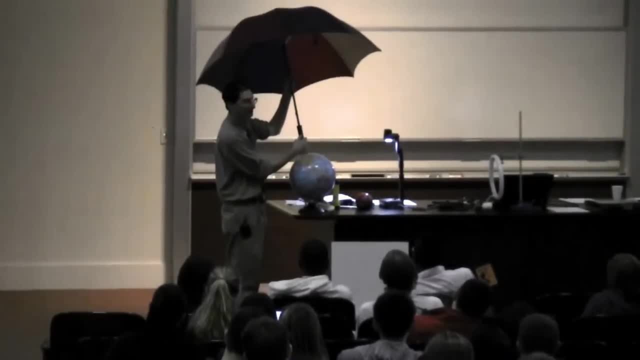 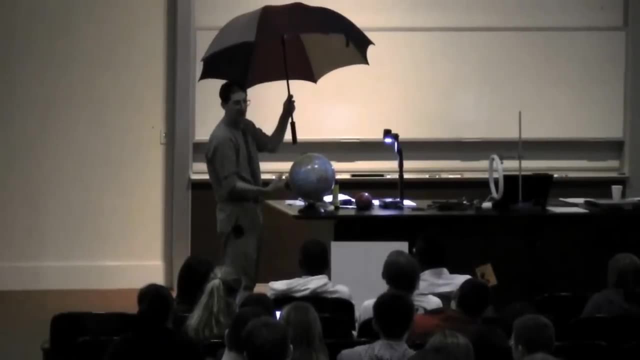 Yes, In fact, there are how many points? Two points, That's right, And so we call them not the North Pole and the South Pole, but the North Celestial Pole and the South Celestial Pole, To distinguish it from the North Pole, which is where Santa lives, and the South Pole down. 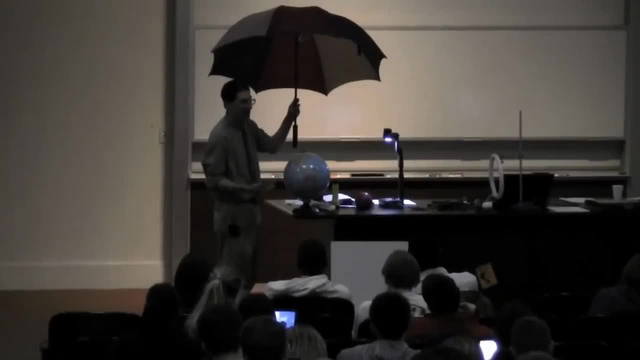 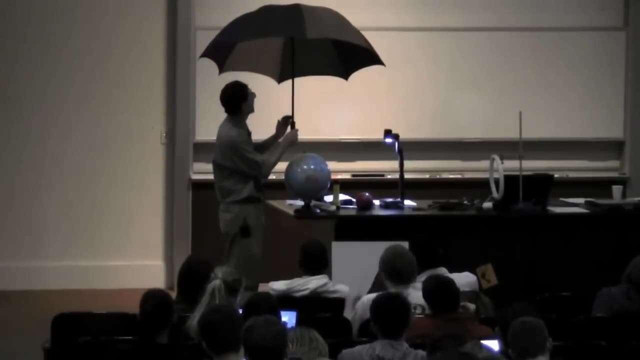 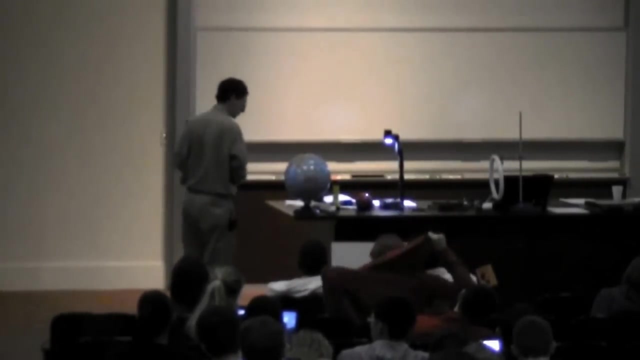 here North and South Pole of the celestial sphere, And really it has nothing to do with space. it's just an extension of our particular planet's rotation axis, out intersecting this imaginary sphere that we believe all the stars are painted on. So let's write down those terms. 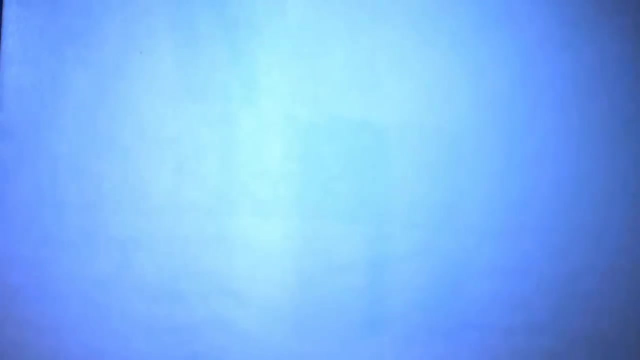 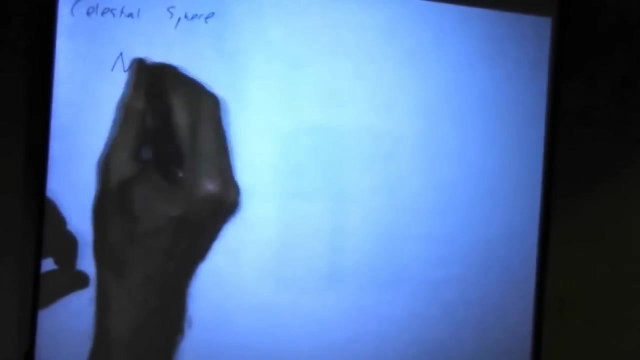 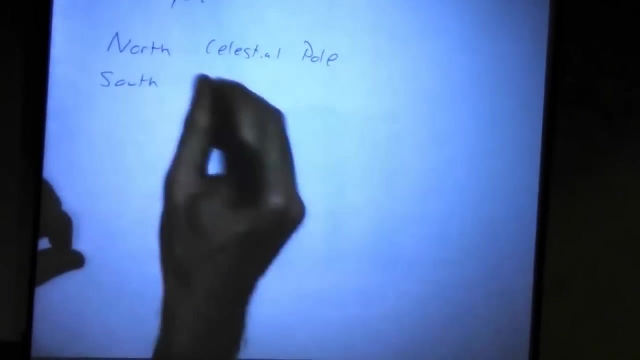 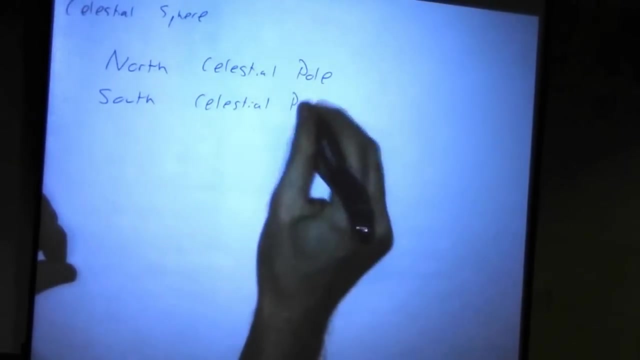 Okay, Celestial sphere. So we have the North Celestial- Okay, Celestial pole And we have the South Celestial Pole, which is just an extension from through Earth's rotation axis, through the South Pole, out to the idea of the celestial sphere. 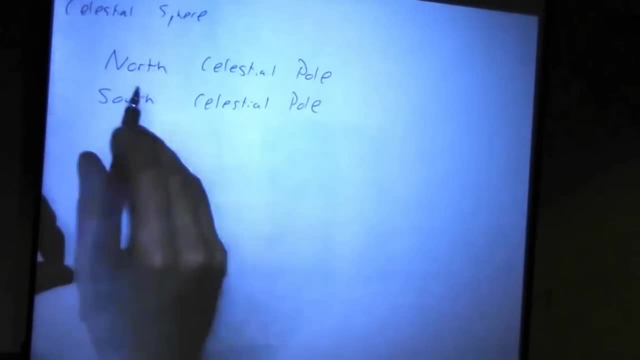 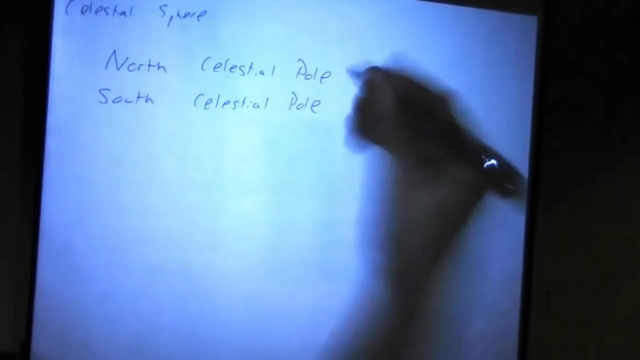 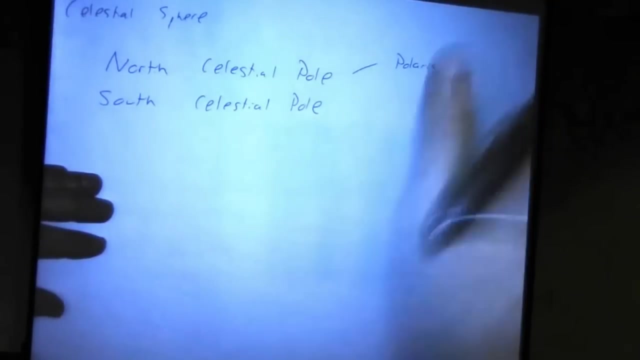 Now there's a star very close to the North Celestial Pole. what do we call it? Polaris? Polaris, yes, Sometimes it's called the North Star. Its technical name is Polaris, And so it's again along the pole of Earth's rotation axis. continue out in that direction. 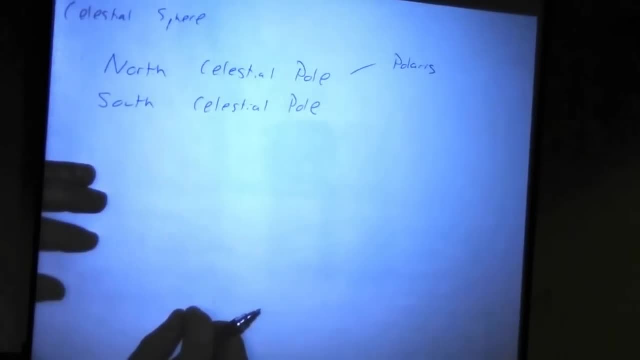 and we have a star. It's not exactly at the North Celestial Pole, but it's very close and it's relatively bright. If you go faint enough, you'll find something close enough to either celestial pole, But it's relatively bright. 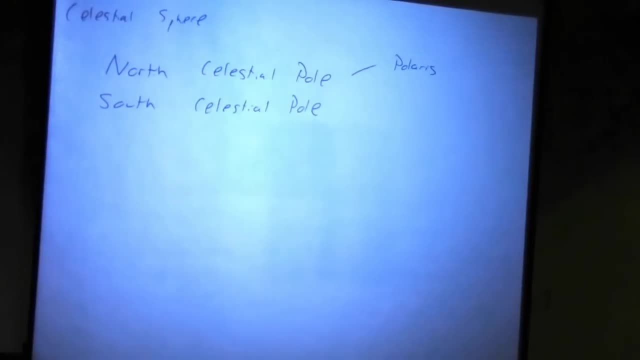 Now, if you're looking in Chapel Hill, if you go out looking for the North Star, looking for Polaris, it's hard to see in Chapel Hill. It's bright compared to the North Star, The vast majority of stars out there, But it's kind of faint compared to what you can see with the human eye under city conditions. 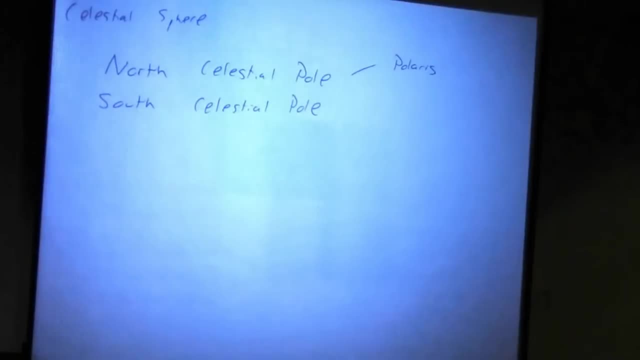 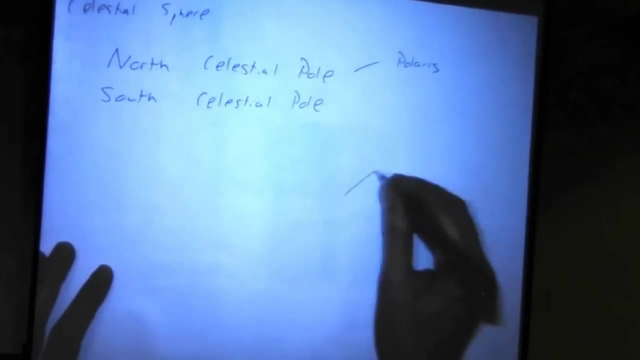 If you go outside of the city, particularly on a moonless night, you should have no problem seeing it. In fact, it's easy to find. This is kind of total tangent, not where we need to go, But one of the easiest things to find. I said we're not going to learn constellations, but 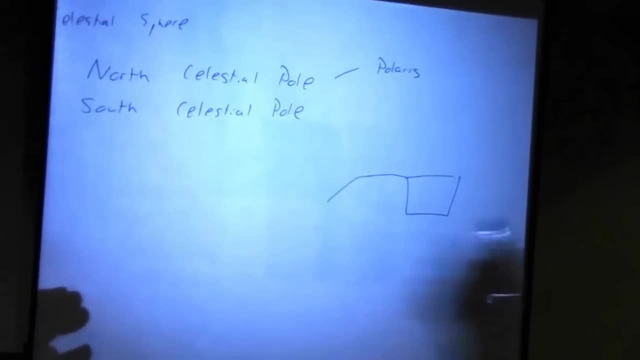 I can't help myself. One of the easiest things to find in the sky is the Big Dipper. So here's the Big Dipper. If you take these two stars from the Big Dipper and just continue off into the North Celestial Star, and just continue off in that direction, you'll find a fainter star. 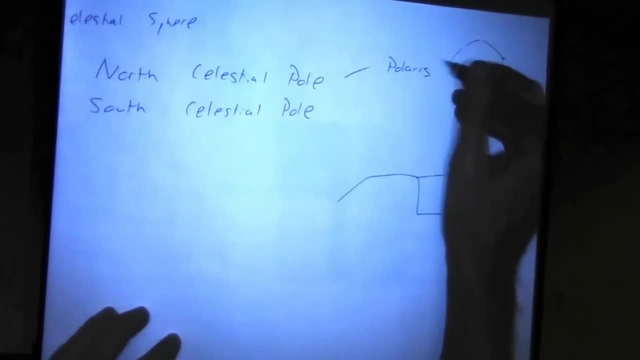 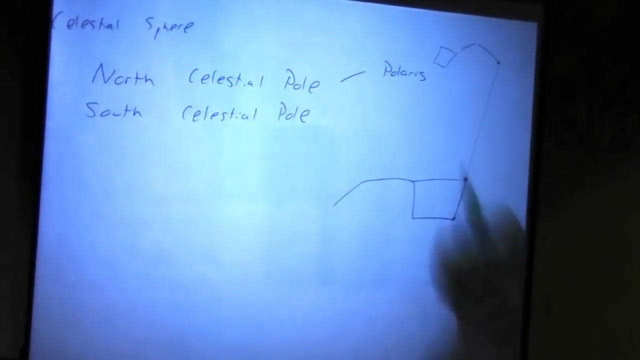 And it's actually on the end of the handle of the Little Dipper. The Little Dipper is sometimes hard to see because some of the stars in the Little Dipper are very faint And if you're looking in the city it won't look like the Little Dipper, because you won't. 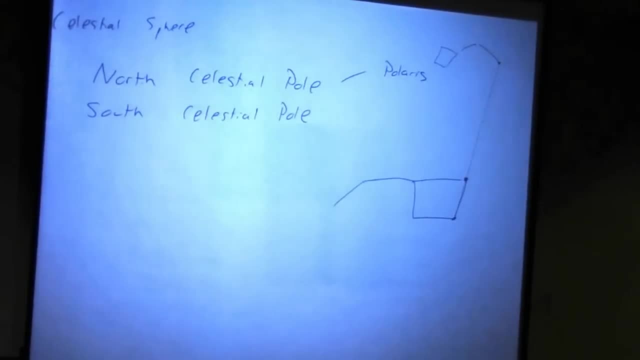 see them, But you might be able to see Polaris under city lights, And that's how you find it. If you're having a hard time finding it, another trick is to line yourself up on street grids. Streets are normally north, south, east, west. 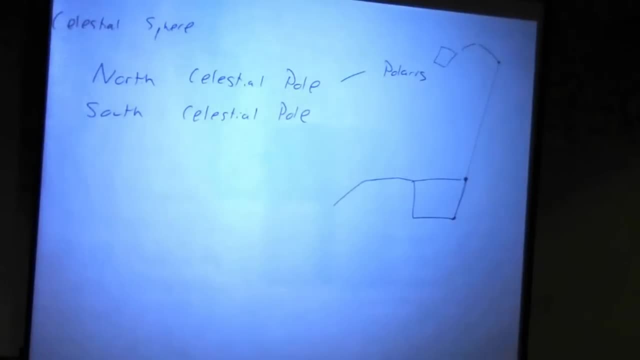 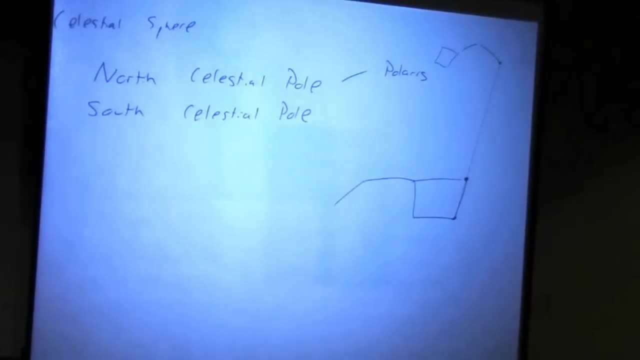 Just follow the street and look up and you should find it as well. Anyway, it was used going back through history to help navigate ships. You know you're out at sea, which way is north, while you find that star and that star. 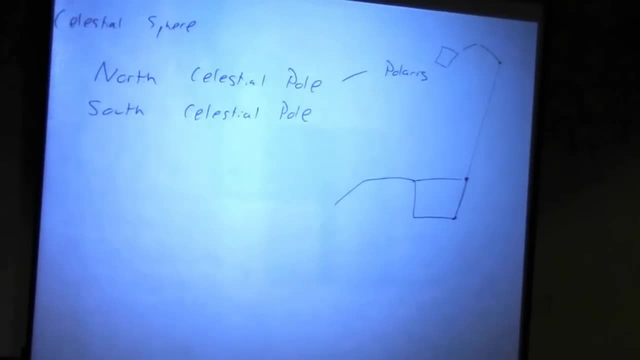 is always there. It's not moving like the other stars. You latch on to any other star. it's moving in the sky, Not very good for navigation, but there's that one star that's always there, at least when the sun is down and the sky is dark enough. 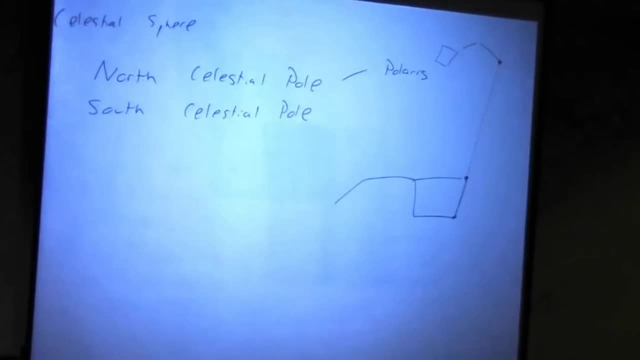 So it has a unique place in history. but we'll see, It's not always there. It moves, It's not always close to the North Celestial Pole. Let's see here. Okay, here's a question. If we were standing on the North Pole of Earth, where would the North Celestial Pole be relative? 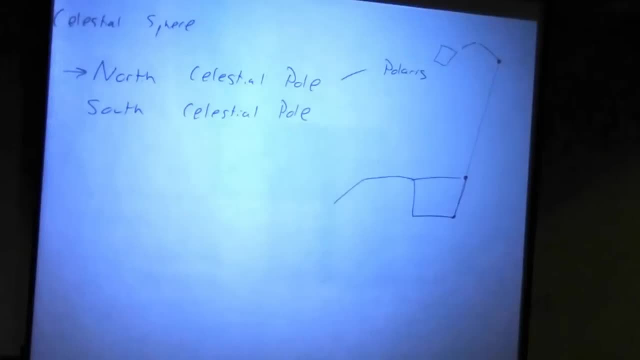 to us, To our left, to our right, up right, straight overhead, Because the North Celestial Pole is an extension of our rotation axis. if we're standing on the North Pole, imagine a little person standing here. they'd have to look directly overhead. 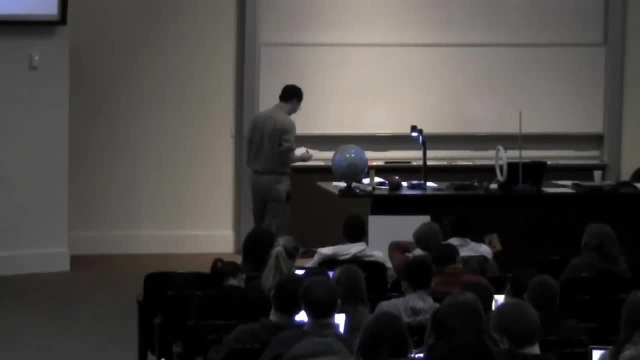 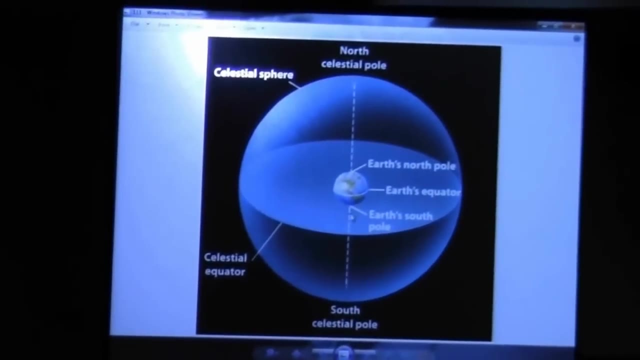 to see Polaris, So Polaris would be up there. So let's see, I've got a figure here kind of shows that Here's Earth and here's its rotation axis, extended out to meet what we're calling the celestial sphere. 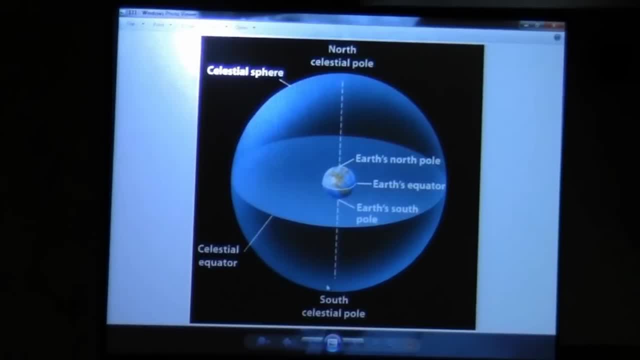 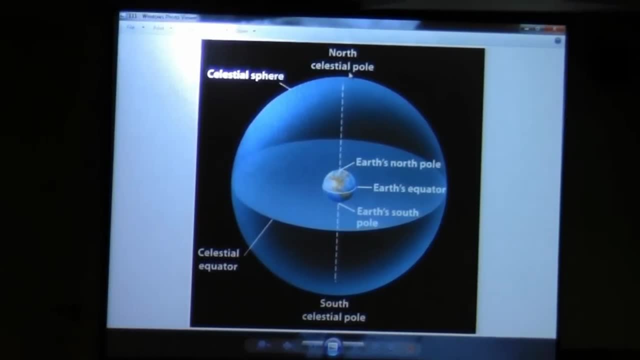 Again, envision all the stars painted on it. Here's our North Celestial Pole, South Celestial Pole, So you can envision standing there. You'd actually have to bend your head all the way over and look up to see the North Celestial Pole, to see Polaris. 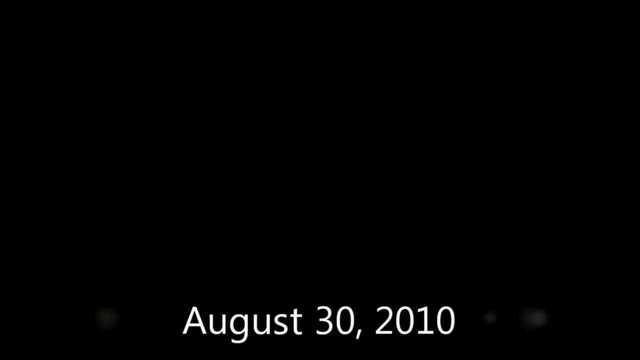 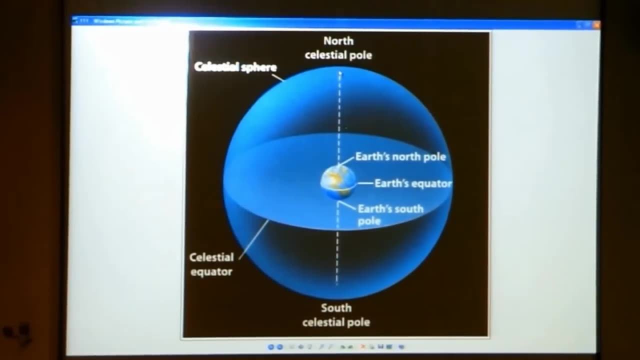 But we're not on the North Pole. we're here in North Carolina. granted, North is in both names, but it's not the North Pole. We're partway down on the Northern Hemisphere. so is that North Celestial Pole still straight? 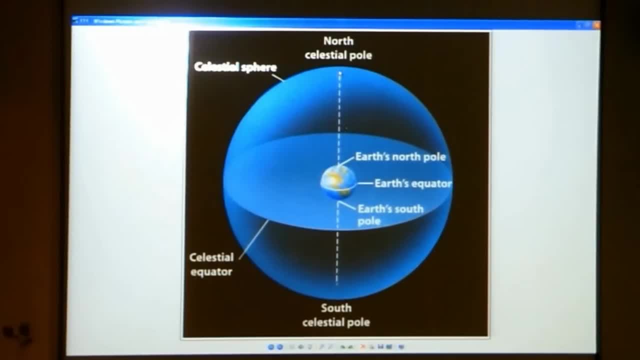 up. No, Remember, we oriented the room north, south, east, west, to go ahead and point to where the North Celestial Pole appears. The North Celestial Pole appears in our sky, That's right, it's partway up the Northern Hemisphere. 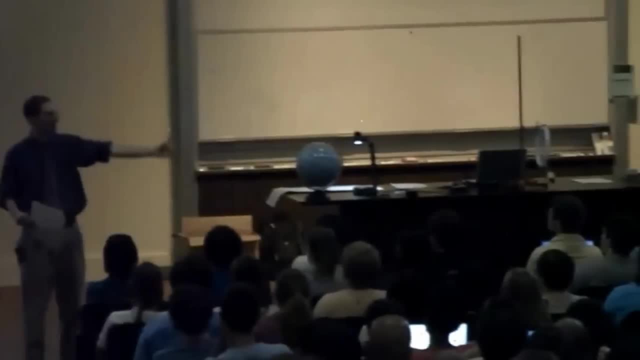 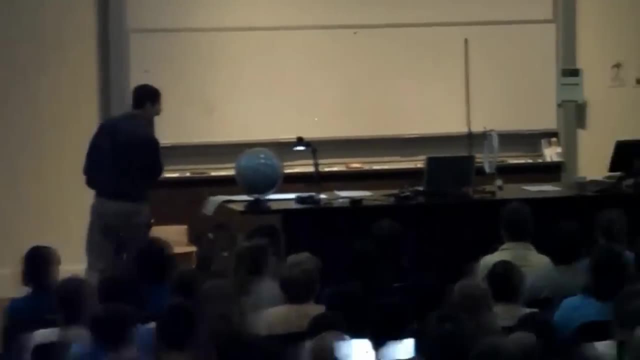 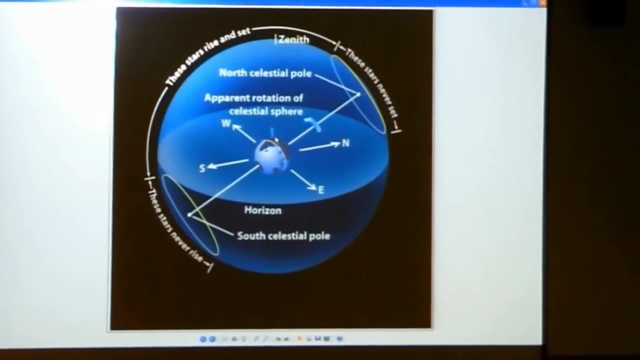 The farther we go down to the equator, the closer it gets to the horizon. So I'm going to bring up another image that might help to illustrate this. So here, same kind of figure, except it's tipped over. Here we have the Earth. 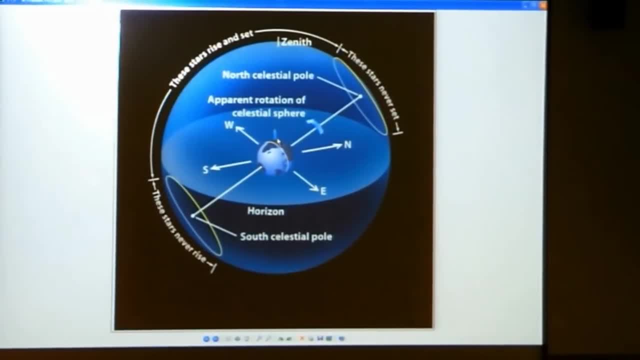 Here we're standing, I guess, in North Africa or Southern Europe, but that's kind of, you know, rotate the Earth a little bit. it's like you're standing in North Carolina, Pretty close anyway. And so here we are. 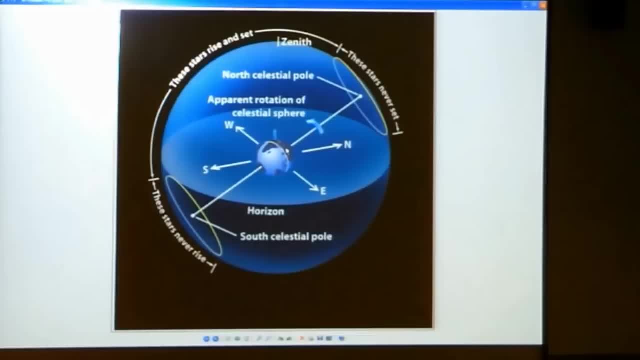 And so here's the line going through the rotation axis of the Earth- North Pole, South Pole- you can see it well here- and where it intersects with the fictitious celestial sphere which gives us our North and South Celestial Poles. 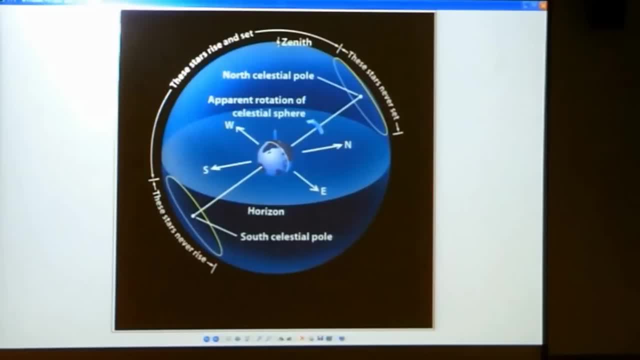 Now the point: directly overhead. in terms of terminology, we call that zenith. That's a term that we'll use. Zenith means directly overhead. It doesn't mean directly overhead the North Pole. it means directly overhead of wherever you are, But indeed it's not directly overhead. 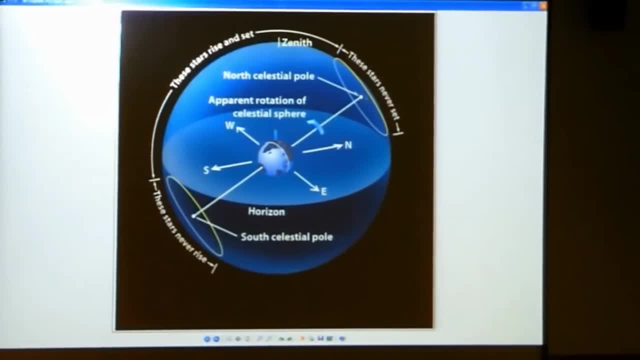 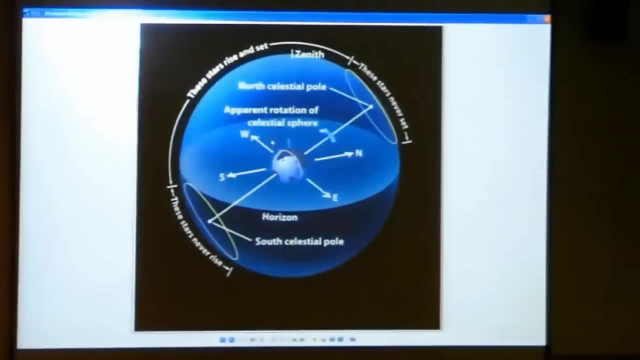 It's not directly overhead the North Pole. It's not directly overhead the North Pole. The North Celestial Pole is not up here at zenith, like it would be at the North Pole, but down here in the northern sky. Here's north, south, east and west, so it's in the northern sky, closer down to the horizon. 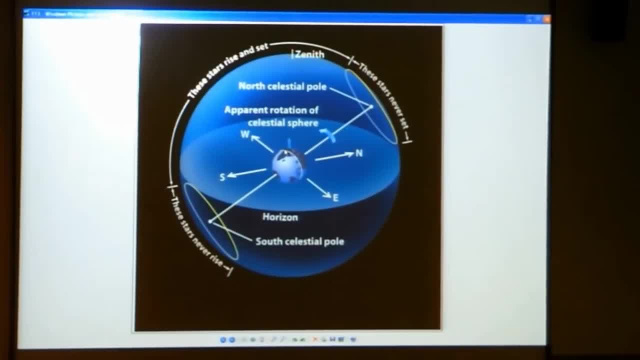 If you keep moving down farther to the equator, then the Earth is tipped on its side, and so the North Celestial Pole will be on our horizon. So if we're near the North Pole- it's up there- we start marching down towards the equator. 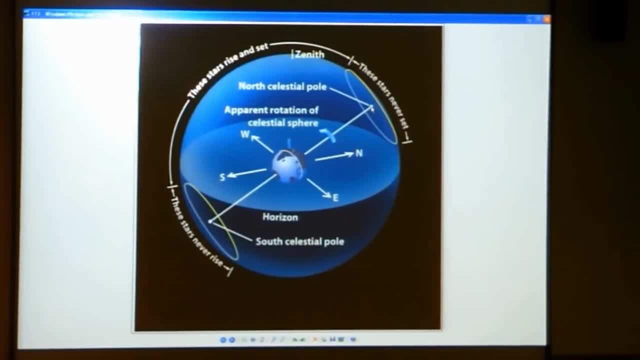 it moves down and, down and down until it's on our horizon and all the stars will be going around it at that time. Now, this introduces some extra terminology here, and these are called, in particular, groupings of stars, called circumpolar stars. 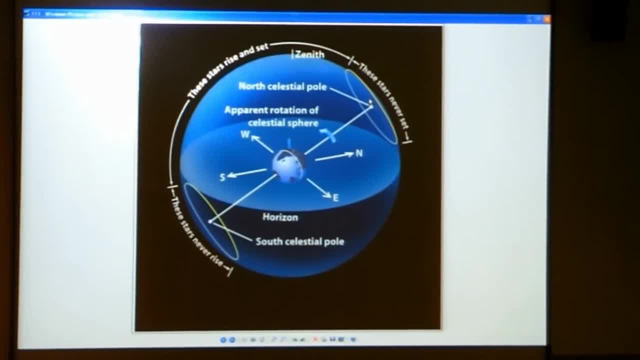 These are stars that never set or never rise around the two poles. You can see a mark here. There's a circle on this diagram going around here. So if that's a star, it's going around, it gets high in the sky, comes down, gets up. 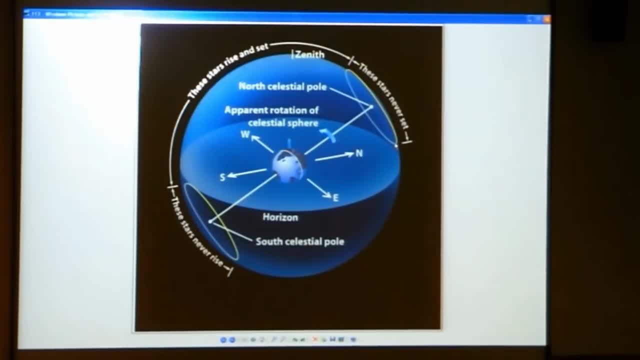 and then it goes down. So it's close to setting but doesn't quite set. And everything interior to it closer to the North Celestial Pole will be the same deal. It will move around the North Celestial Pole, but it's a small circle and it pulls high. 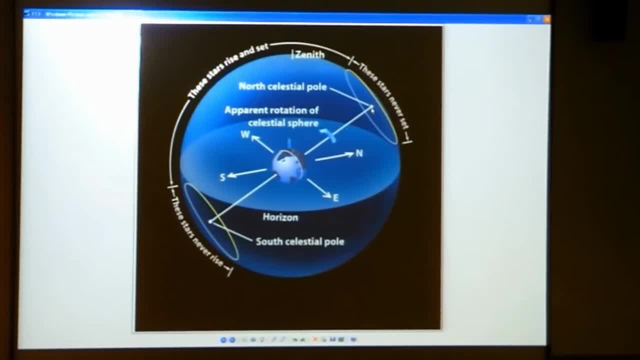 enough off that it never sets. So there are some stars that never set. You call it a circumpolar, And down in the southern celestial, in the southern sky, around the southern celestial pole, you have stars there that never rise. Anything within this cap we can't see from the northern hemisphere. 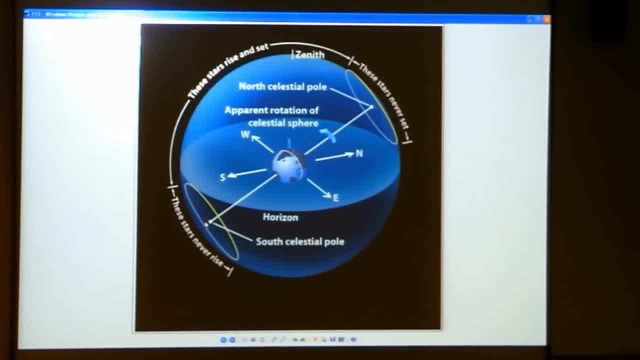 The stars are always below the ground. It makes sense. We're in the northern hemisphere, We're not going to be able to see part of the southern sky because the Earth is in the way. So those are circumpolar stars. That make sense. 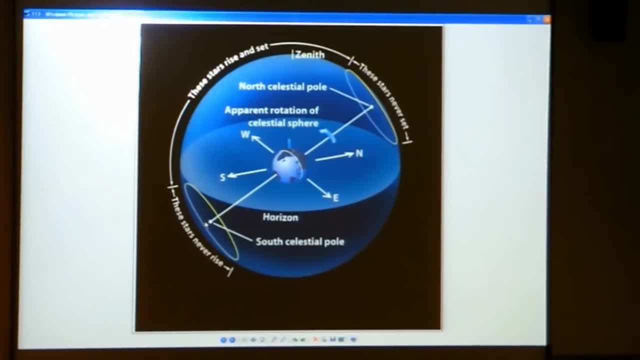 Question: Well, if you're on an equator, you can't see all the stars in the sky. That's right. In fact, I just answered one of my upcoming questions. But yes, indeed, If you're on the equator, you can see all the stars in the sky, except, of course, when the sun comes up. When the sun comes up, it scatters its light all throughout the sky and you can't see the stars anymore. So I'd wait six months. You can't see all the stars in the sky, But if you're on the equator you can see all the stars in the sky, except of course. when the sun comes up. If you're on the equator, you can see all the stars in the sky, except, of course, when the sun comes up. When the sun comes up, it scatters its light all throughout the sky and you can't see. 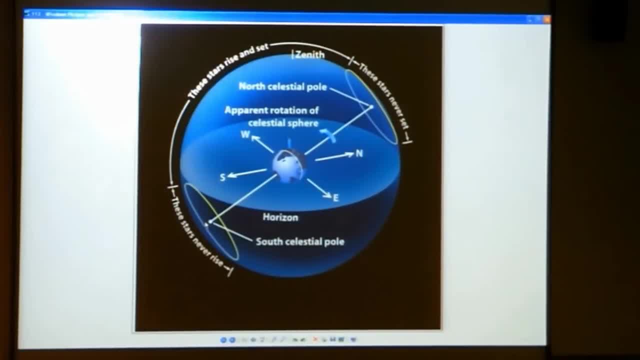 the stars anymore. So I'd wait six months, and then the other set of stars will pop up. Okay, A couple of questions for you, one of which was just answered. But if we were at the North Pole, which stars would be circumpolar? 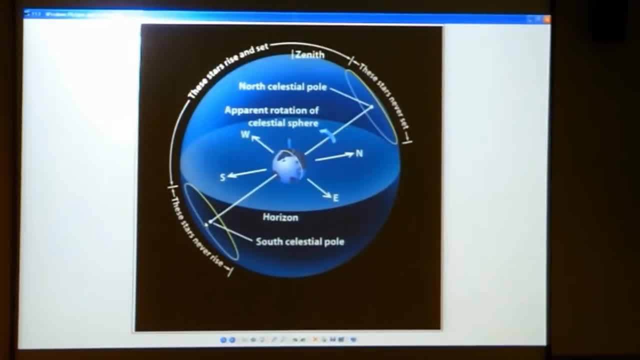 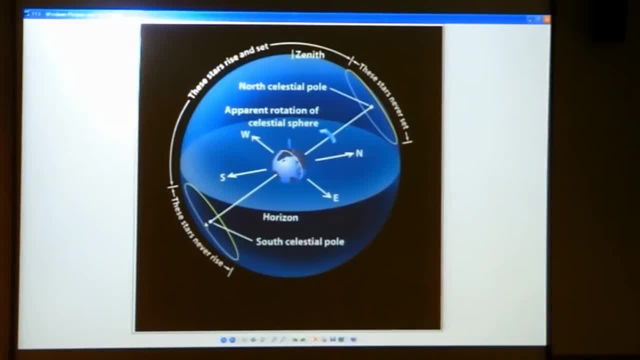 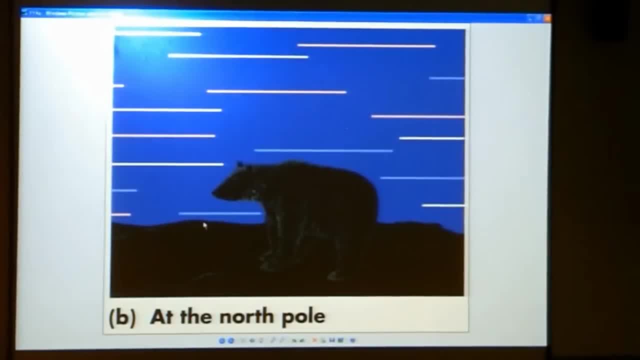 I'll come back to that. So yeah, there's the polar bear that I mentioned. Since all the stars are going around that point directly overhead, as you extrapolate that down to the horizon, they're going sideways along the horizon. All those stars never set. 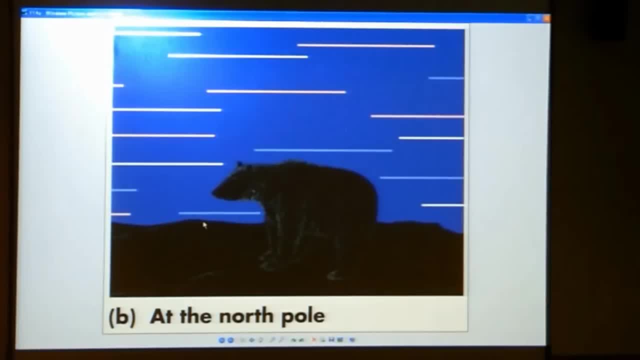 They never rise. They're always above, And when you see half the stars in the sky, they're always up, Even when the sun's up. you just can't see them. And the other question which I'm going to ask you now is: how do you see the stars? 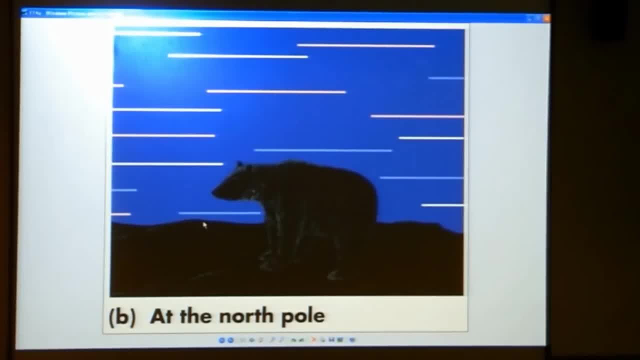 in the sky. How do you see the stars in the sky? How do you see the stars in the sky? All those stars never set, They never rise, They're always above, And when you see half the stars in the sky, they're always up. 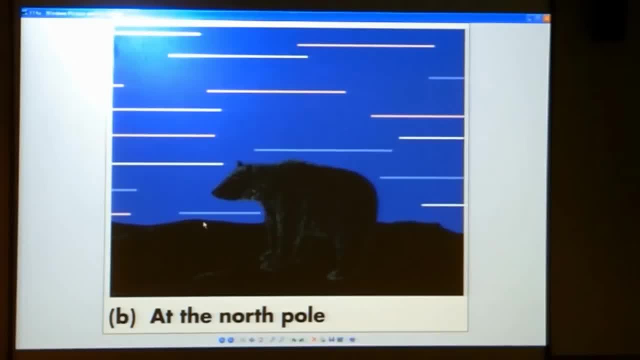 Even when the sun's up, You just can't see them. And the other question which was answered there: if you're standing at the equator, what fraction of stars are circumpolar? And the answer is None, None. 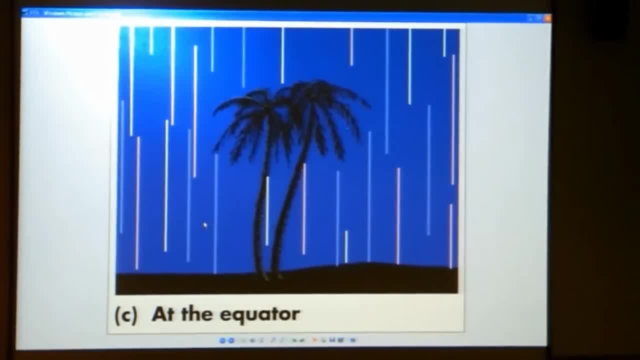 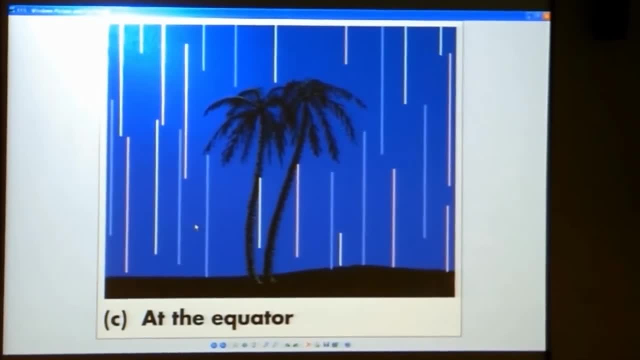 So here we are, at the equator, And remember, if you're standing on the equator, let's see north was that way. So the north celestial pole will be there. The south celestial pole will be there, And maybe this one. 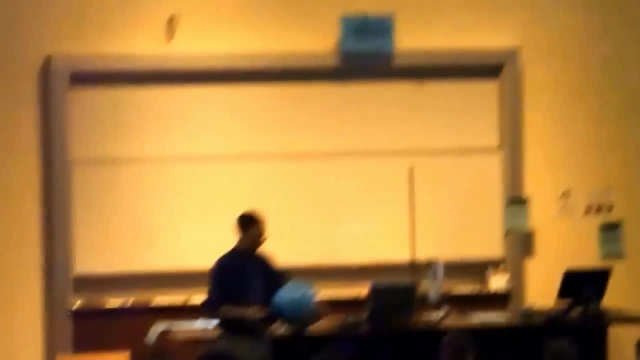 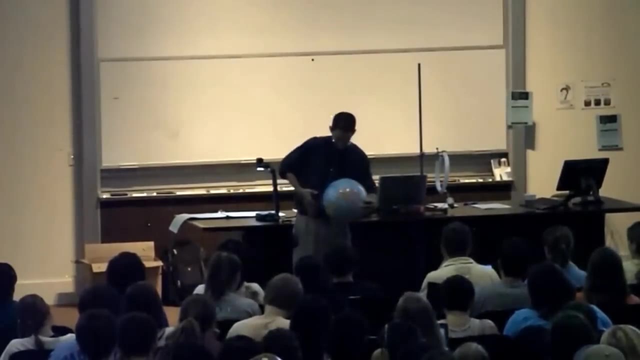 will help illustrate. it will stand on the equator. so here's the earth, here's the equator. as I said, my my screens don't let me touch anything. there's a reason. so if you're standing here on the equator, then the north celestial pole will be. 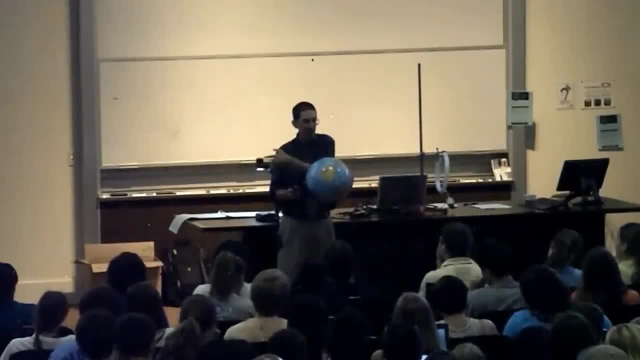 along the rotation axis, in that direction. south celestial pole will be in that direction direction. so here's your ground, your horizon will be there and the stars will come up in the east and set in the west over there. they're coming up in the east, setting in the west west and setting the side sky from. 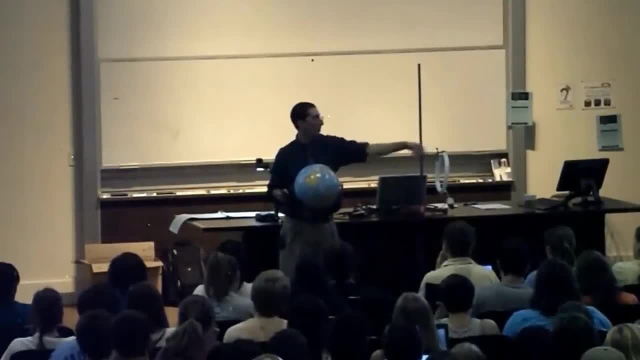 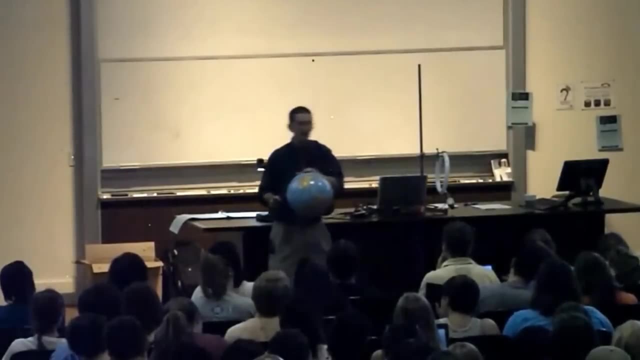 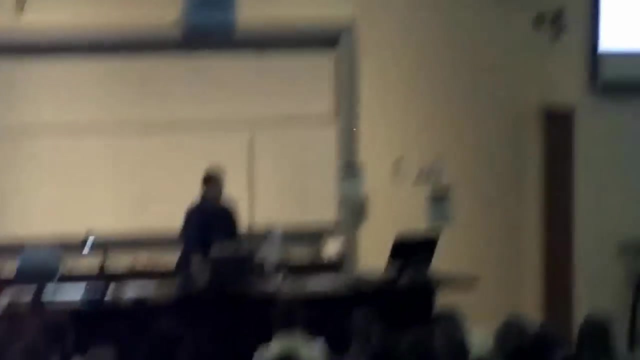 up and east, setting in the west, rotating around those two poles. so all the starts rise, all the stars set. the none of the stars are circumpolar. if you're at the equator, okay. okay, let's go back to this figure. let's skip this. it's kind of cool. 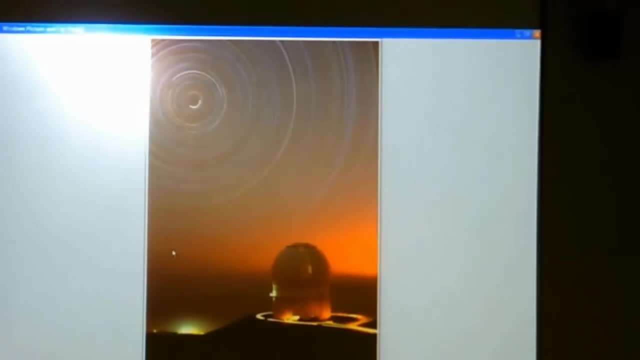 as I'd win the northern hemisphere, because we all agree on, and that means the north celestial pole is not straight overhead but somewhere in the Northern sky. So here's a picture. I'm not exactly sure which observatory this is. I always think it's Kitt Peak, which is near Tucson. 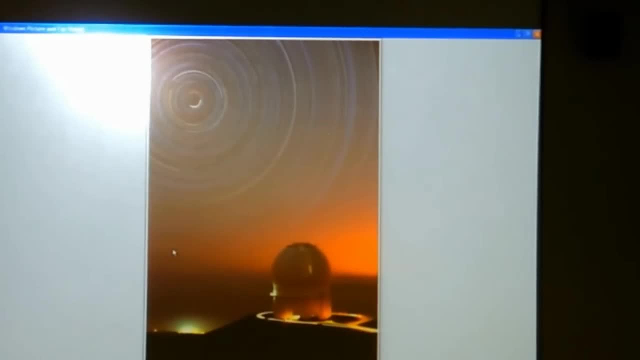 That light in the background is Tucson, but that telescope isn't one of the telescopes at Kitt Peak. Kitt Peak's well in Arizona, near Tucson, Anyway, some northern hemisphere observatory. It might be Mauna Kea in Hawaii. 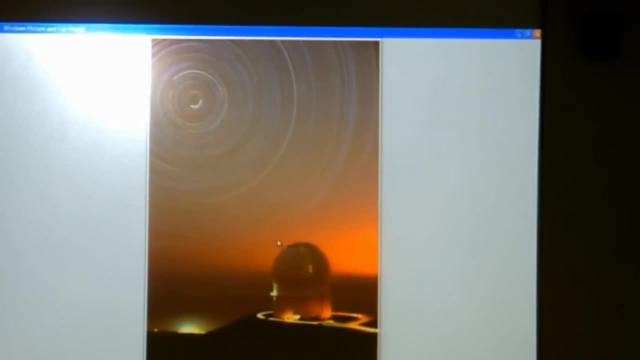 I'm not exactly sure, But anyway, this is a time-lapse photo, And so you know it's actually quite dark, It seems bright, It seems like sunset or sunrise, just because the camera shutter is open all night. Every little bit of light that comes in gets counted and accumulated over the course of the night. 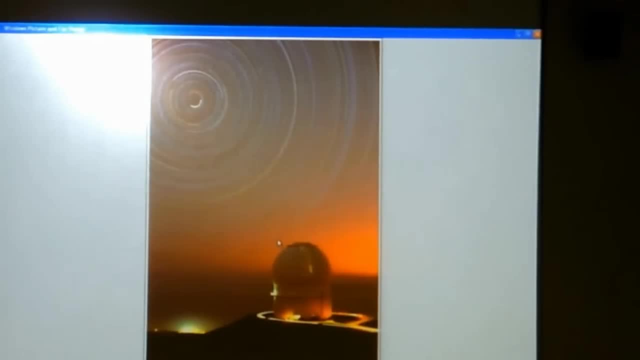 And so you know the camera's sitting on the ground, so the telescope's not moving. with respect to the camera, It's always sitting there. You can see the cars that came in and left over the course of the night, leaving the trails of their headlights in the exposure. 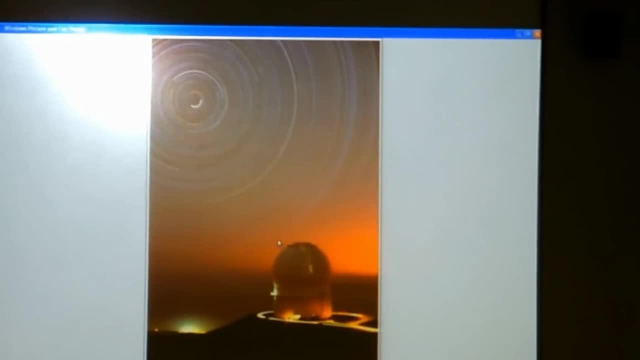 The stars rotate around the North Selection Pole So you can see that motion. there. You can see where the North Selection Pole is. It's hard when you just go out, You know you see stars, You're not exactly sure which one is the North Star. 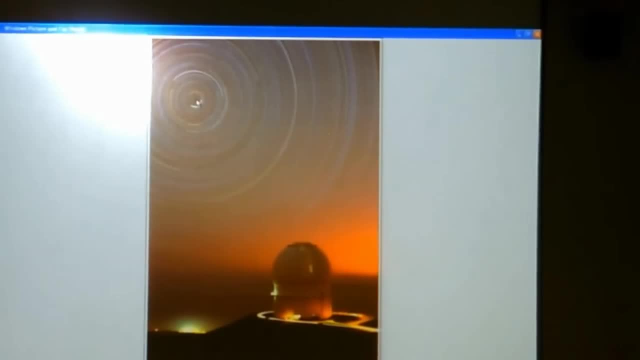 But in a time-lapse photo it's pretty easy, It draws a bullseye for you. So right, there's the North Selection Pole. This bright star is guess what? Polaris. yeah, Now, Polaris is actually kind of hard to see, say from Chapel Hill. 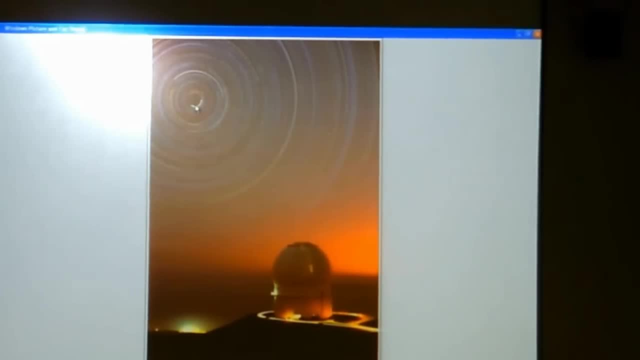 You go out on a good night, you can maybe see it. Or if you get out of the city, You know the moon is down. You can see it pretty easily, But it's a relatively bright star compared to other stars. Most of these other stars you wouldn't be able to see with naked eyes. 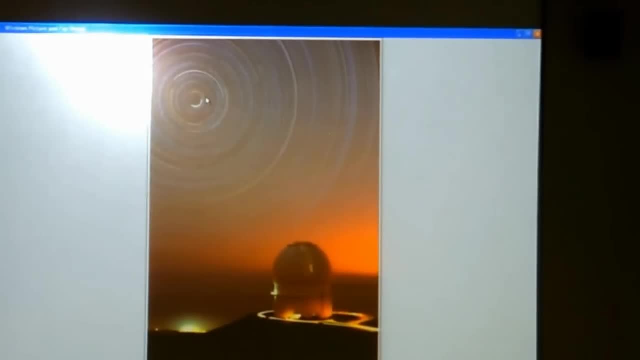 Only because it's being captured on film, Collecting extra photons so that the eye can take it and store it. You can see them. And another nifty thing you can do with this image: you can tell me approximately how long the exposure was. 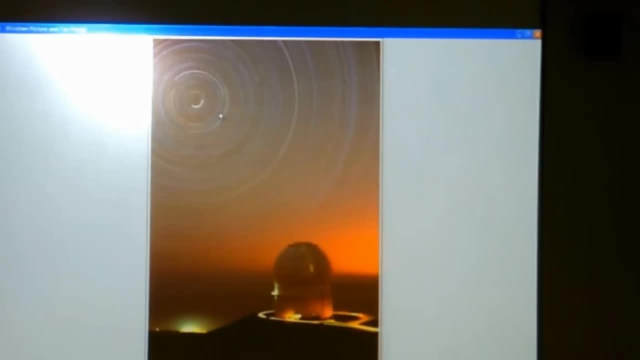 How long they left the camera open. You want to venture a guess About Eight hours? yeah, because a full circle would be 363 degrees. of course It would be 24 hours. A full circle would be 24 hours. 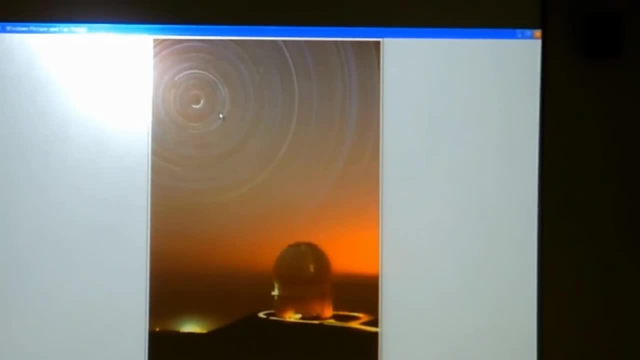 Of course you can't. the image would be pure white because it's the daytime hours, So it's about a third of a circle, a little bit more than a third of a circle, So I'd guess like maybe nine hours. 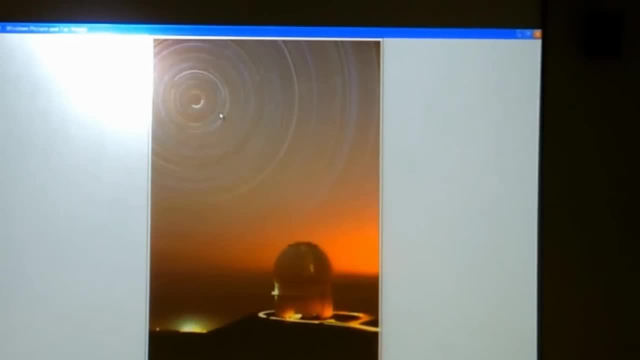 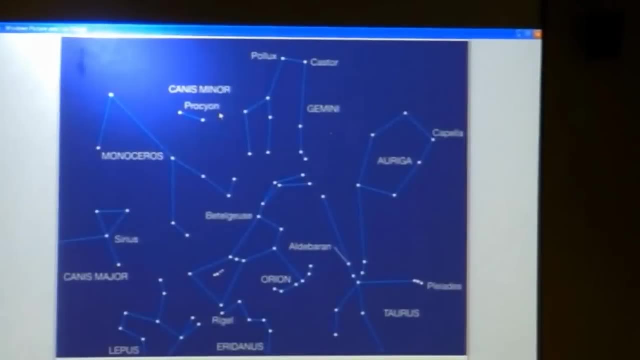 So the sun went down. you had nine hours of night this time of year, And then they finished the exposure before the sun came back up. All right, Any questions about that? Okay, I'll point you to the first exercise Now. these exercises aren't graded. 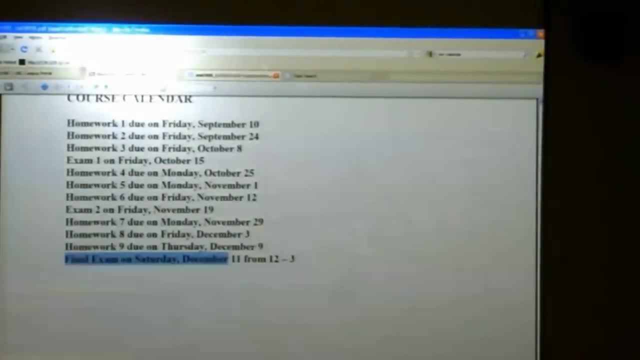 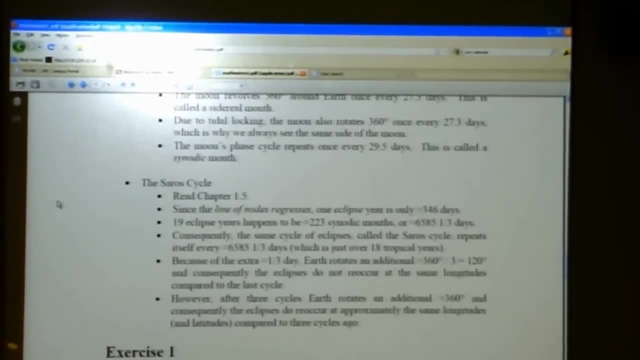 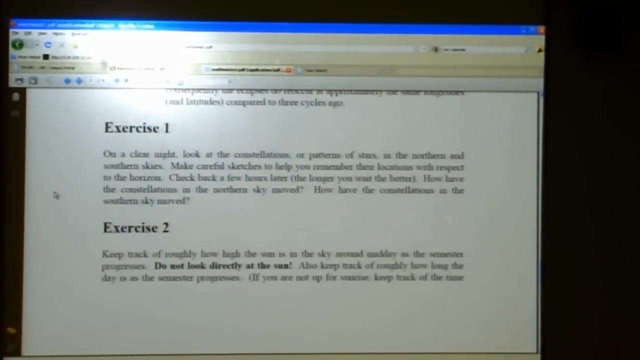 They're just things I'd like you to go out and try to do So. go back to the course homepage. They're all written down in the math notes. If we go down here to the bottom exercise one, Now they're not graded, but you know I can ask you about these on the exam. 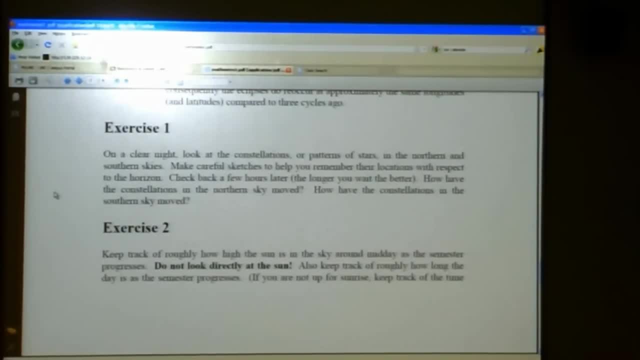 So I encourage you to go out and try it. All right, this one's med-tech convention. So I'm going to give you a sense of what we just talked about: all these motions of the stars. You go out and take a quick look at the sky. you don't see the motions of the stars. 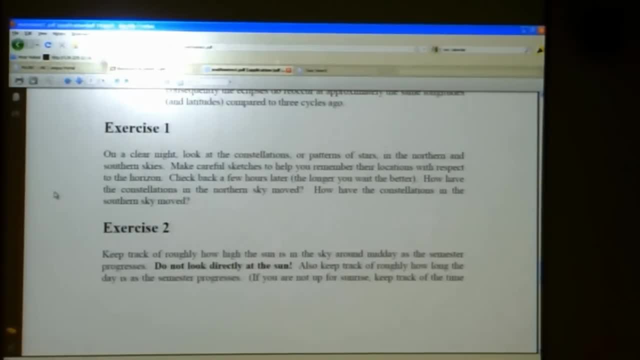 Right now it's just an academic subject in your mind, most likely, unless you've really stared at them for long periods of time. So I encourage you to go out and make a sketch, a sketch of the northern sky and a sketch of the southern sky from some locations, some fixed locations. 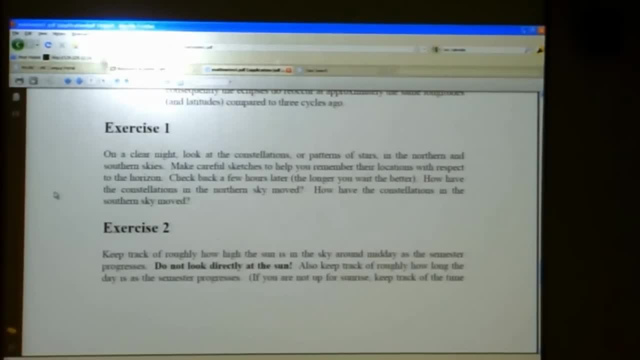 and include some buildings for reference. You know, maybe you have the bell tower over in the south or something like that, And draw, yeah, draw. We start in the sky, but the bright ones, maybe you can identify a few constellations. 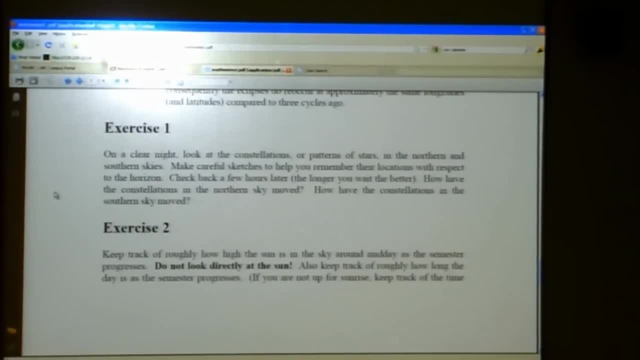 Just draw them with respect to buildings. You know, maybe you do this on Friday night before you go out to have fun. You quickly draw your sketch here, your sketch in the north, and then come back a few hours later giving the sky time to rotate. 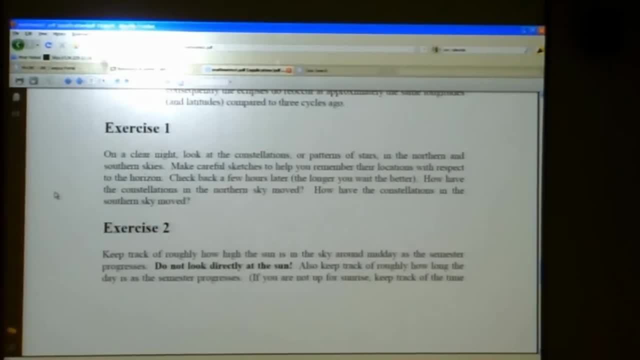 And so, yeah, your second set of drawings might be a little blurry depending on what you're doing, but do it again. And what's your expectation In the southern sky? what do you expect the pattern of stars to do? Yeah, they're going to move, that's right, clockwise, in a broad, sweeping pattern. 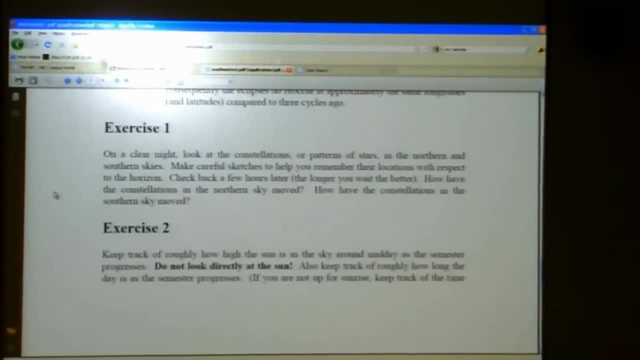 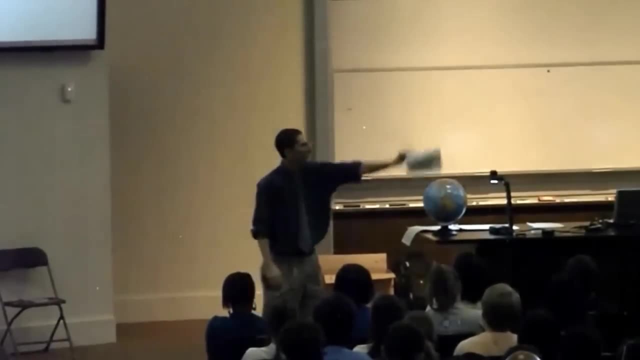 across the southern sky because they're rotating around the south celestial pole, which is beneath the ground. So this is the outer part of the circle, a big, giant circle across the sky. But in the northern sky, what do you expect to see?